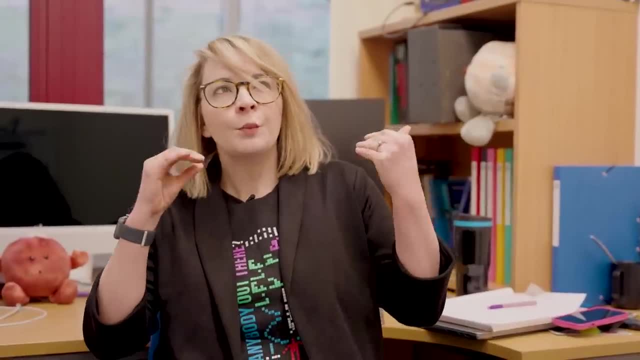 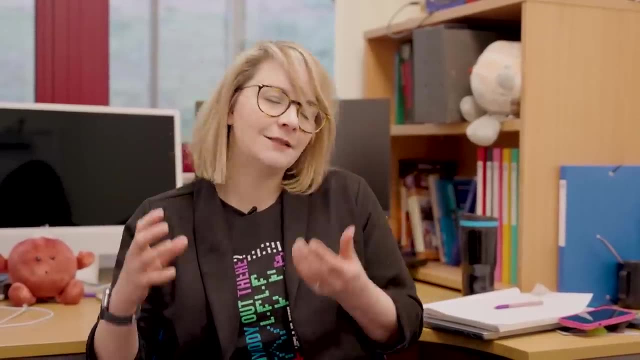 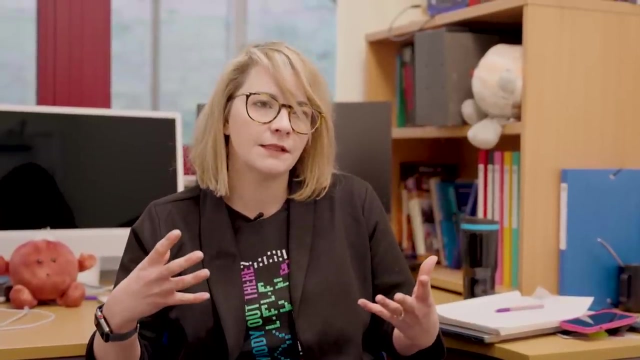 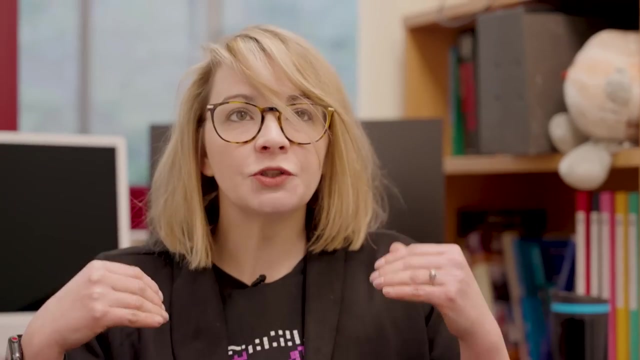 acids on asteroids. That's going to be a moment, But the moment when we realize we are not alone in terms of intelligence, in terms of curiosity and the ability to possibly even talk to a different civilization, that's going to be an existential crisis for the whole of humanity And I'm not sure I want to be there for that. 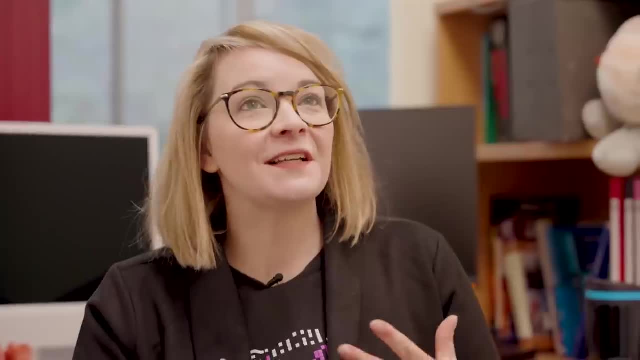 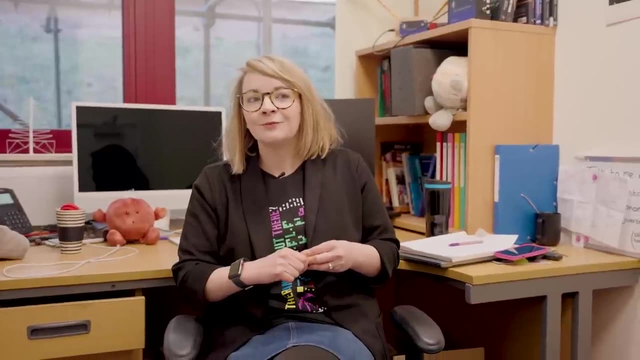 actually I love this field, I love researching it, But I kind of almost don't want to know the answer because I'm not sure humans are going to deal with it very well. Do you want to know what Brady thinks? I want to know what Brady thinks. Brady, what do you think? 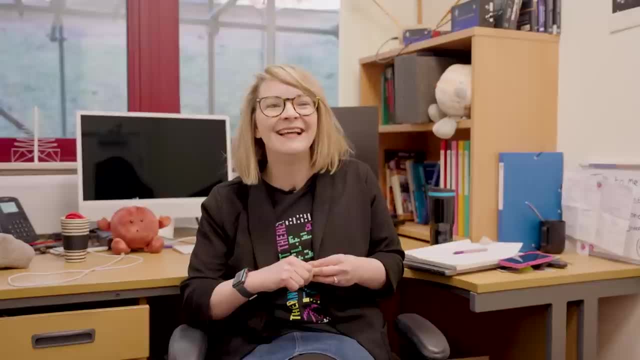 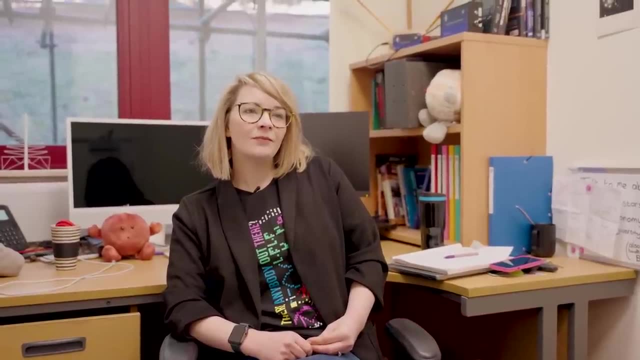 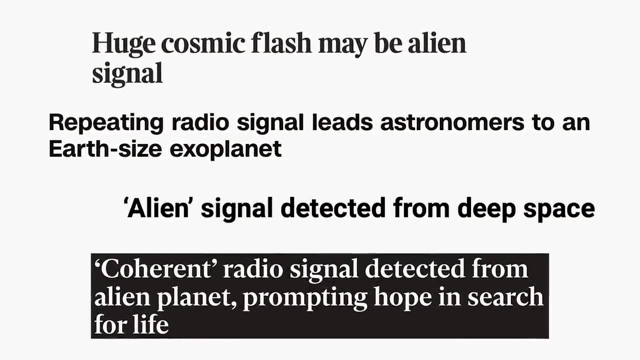 No, it doesn't matter what Brady thinks, because the videos aren't about me, But I'm going to tell you what I think. I think it's going to be a gradual drip, drip, drip of press releases and things like that. that it's maybe, this, maybe, that It could be, could be, And I think by the time we get to the 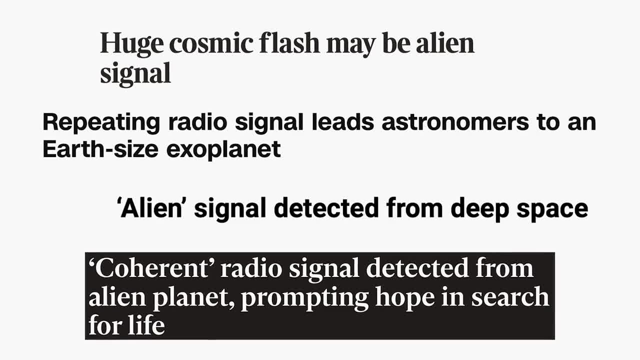 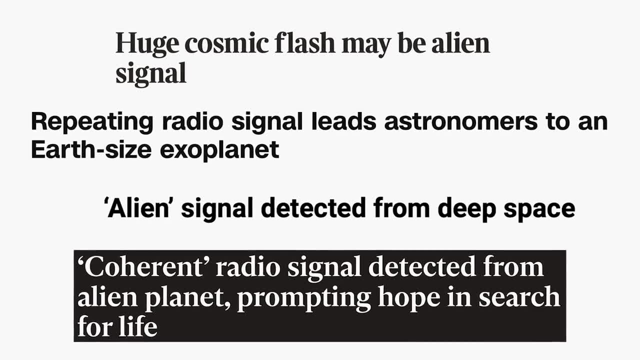 point where we believe it's real. we're going to be so inoculated that it's going to be like: oh yeah, it turns out there are aliens out there and this is where they live on this exoplanet really far away. 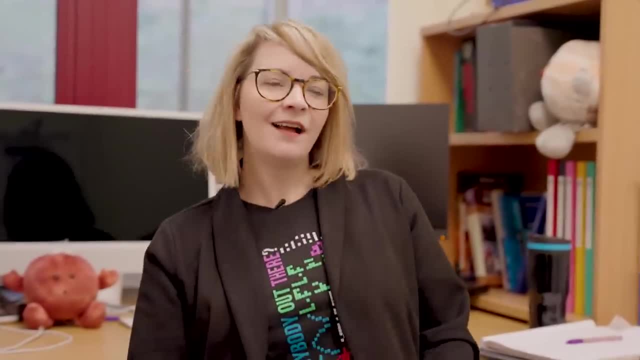 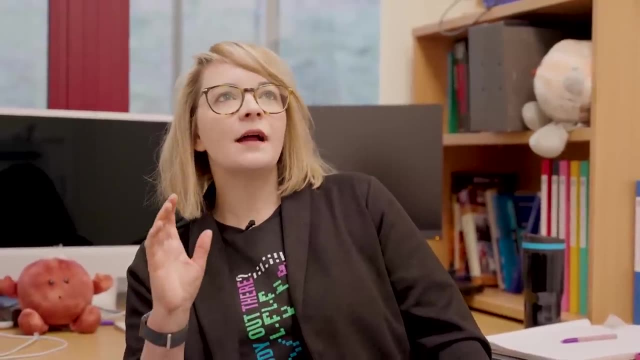 I disagree. I don't think it's going to be the existential crisis you think. I think people are going to be like by the time, By the time we confirm it, I think it's going to be meh. And I think that there's going to be an element of that, because extraterrestrials are so woven into. 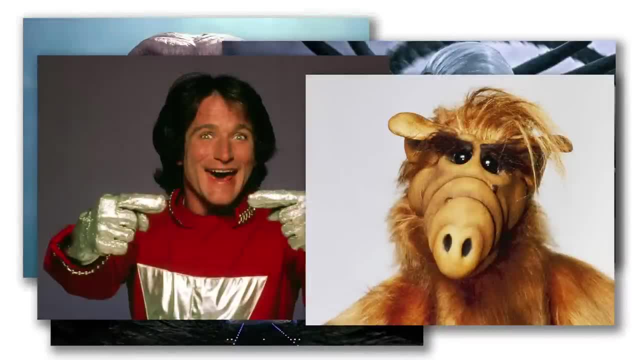 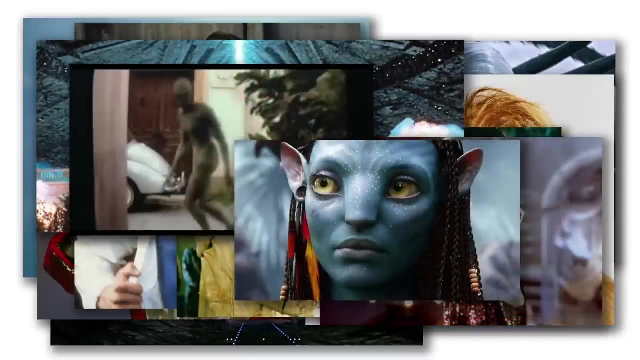 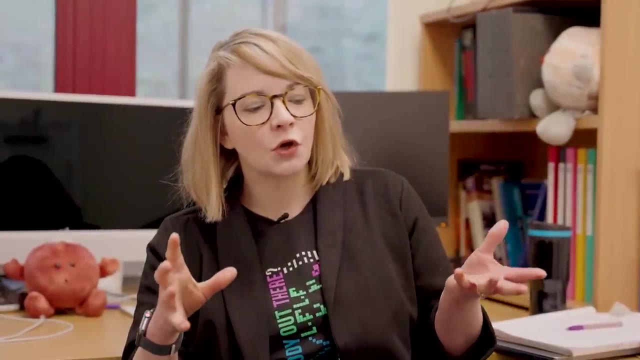 our society and our science fiction and our books and everything. there's all these different types. So I think that that realisation isn't going to be so hard, But I think that because our telescopes, now the way we're searching, is so sensitive that 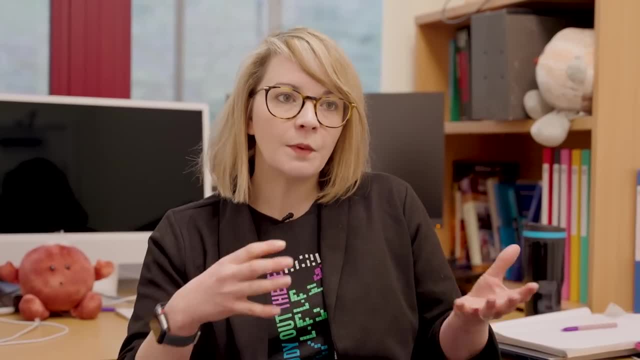 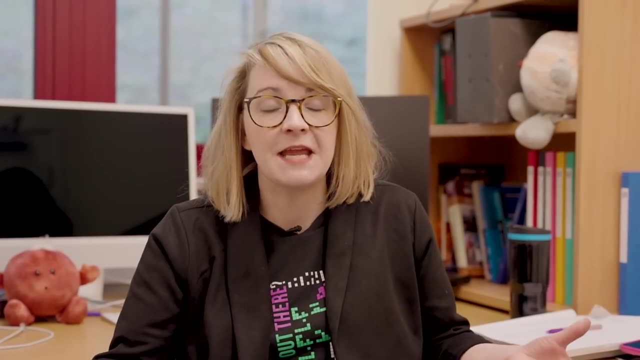 unlike, for example, my work in cosmology, where we're looking for this tiny, unknown signal under a huge amount of rubbish and we're going to, and that's going to be 10 years of like. was that a signal of a first? 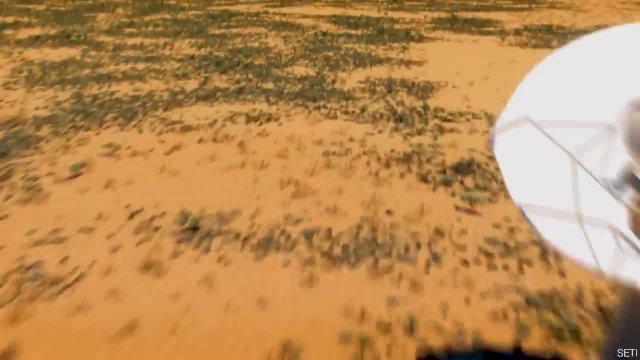 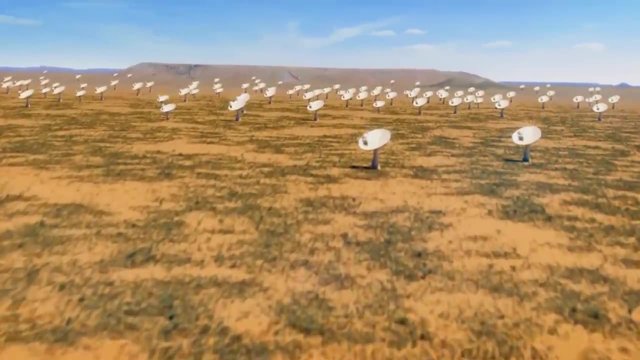 star. I really think that, for example, with a square kilometre array, we switch that on, in a few years we're going to be able to hear the equivalent of an airport radar on a planet 10 light years away very easily, And so there really is the chance here that that it's something like. 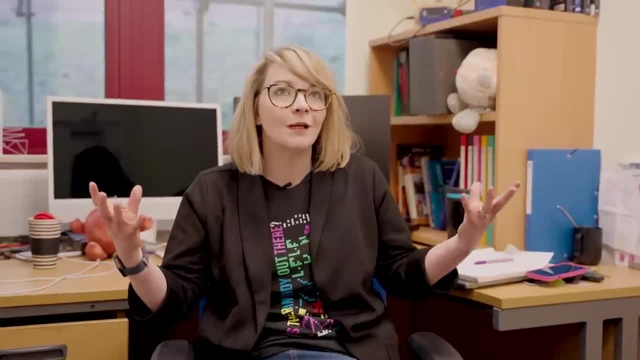 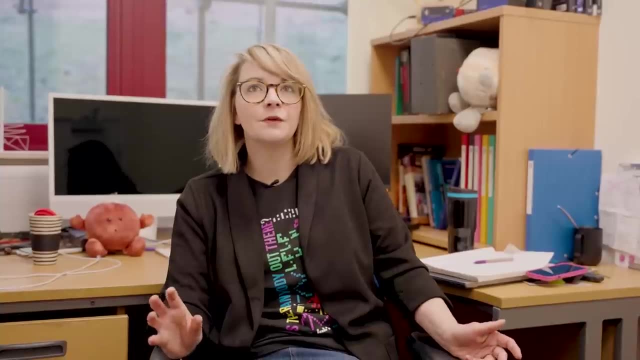 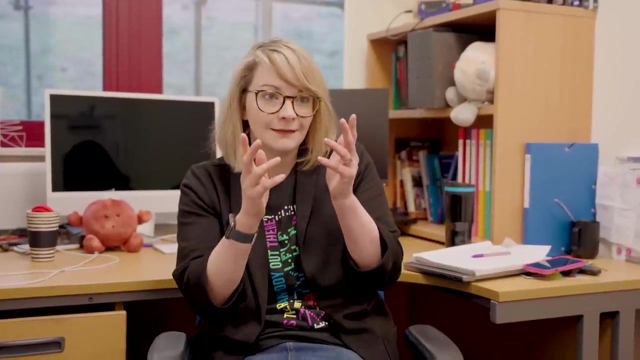 the digits of pi. that is a universal number and will get sent out and it will be really quite clear. There are quite a few ways of checking this signal very quickly by, for example, looking at the planet and then looking away: Is it still there? 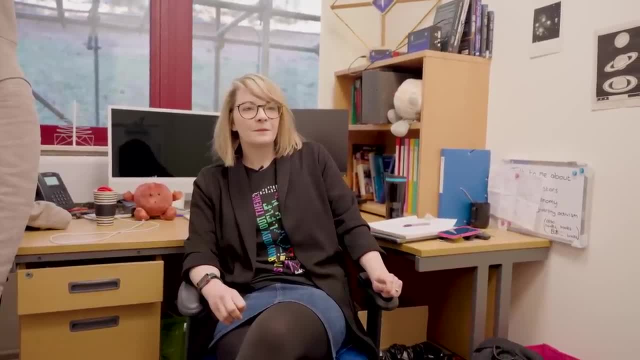 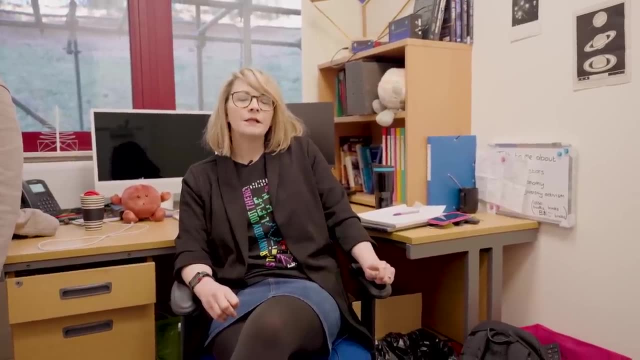 I just think, in the immediate news cycle and our need for immediacy these days, the fact we're not going to be able to communicate with them. Yes, And it will just be. oh yeah, there's a signal there, there's something going on there, but we can't talk with them. 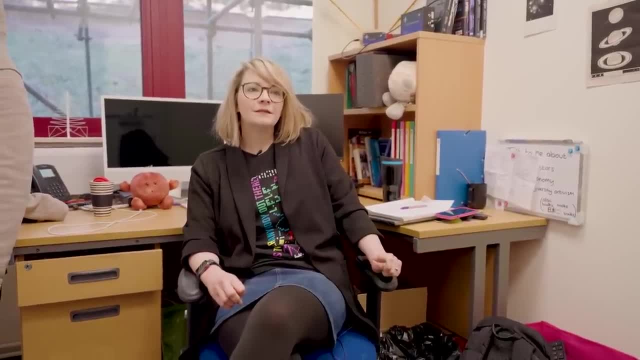 for another five minutes, 500 years. I think people will just be like, well, it's not my problem, I agree with you. I think I think there's going to be a very quick panic of kind of: oh my gosh, are they going to come? 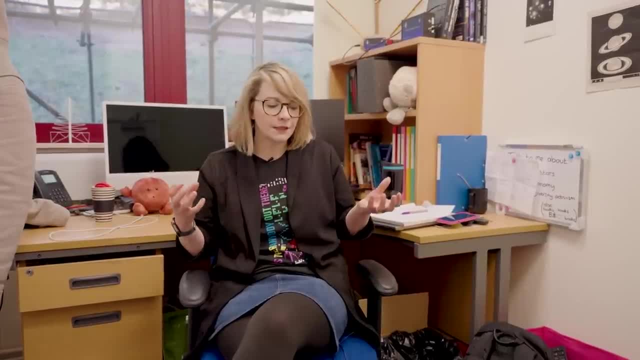 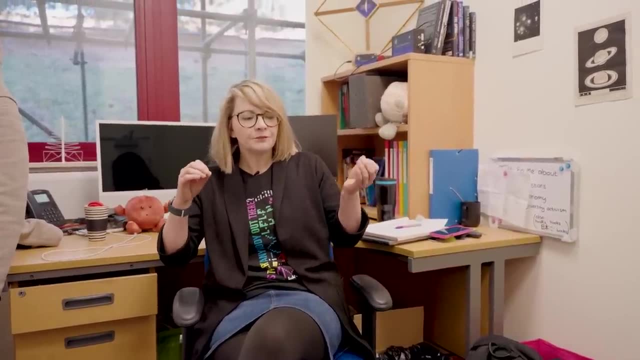 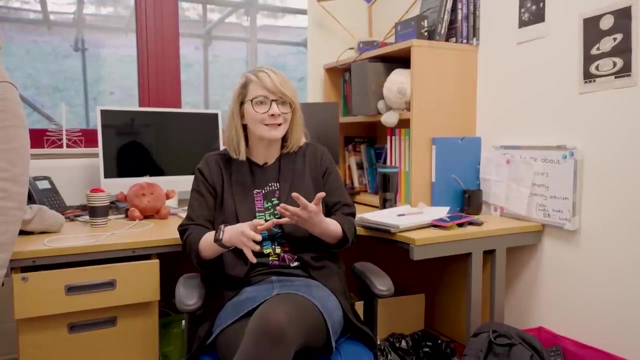 And then hopefully the scientists will be on it enough to communicate- Science- communication is very important in this- that they're not going to arrive here. So to be very clear, anybody in SETI with any credibility doesn't believe that aliens have visited ever and 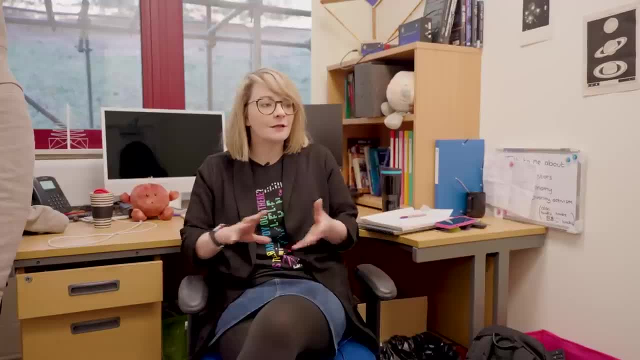 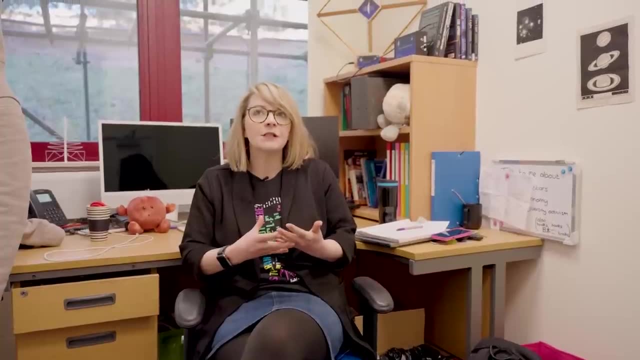 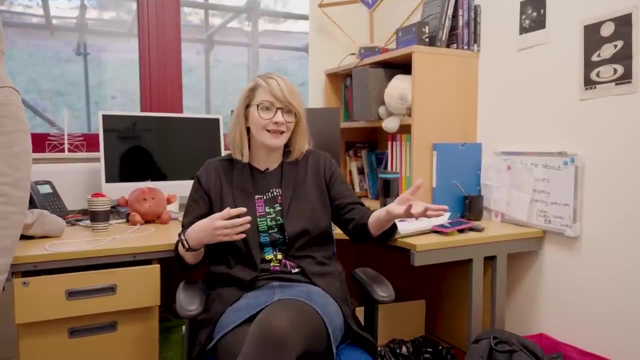 that all the UFOs are there. I mean, if we do start to communicate with these, the extraterrestrial intelligence, they could be 50 light years away or 100 light years away, And so the signal will take 100 years to get there and 100 years to get back. 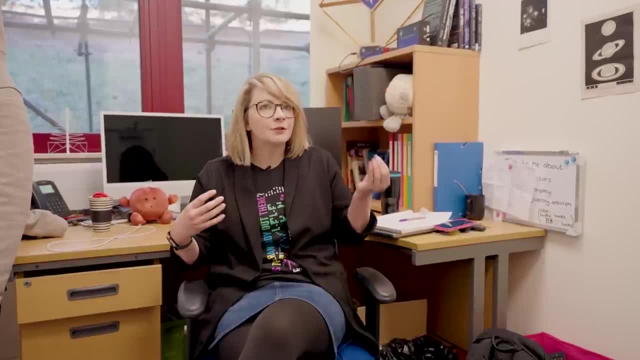 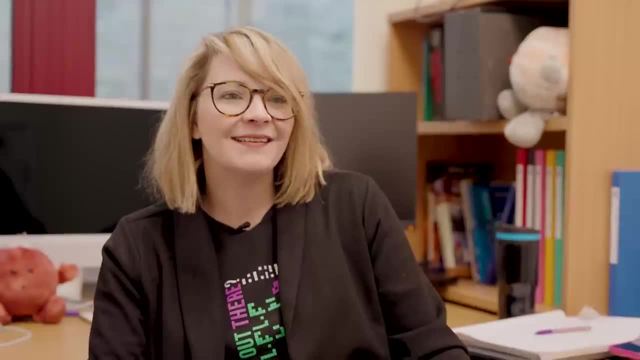 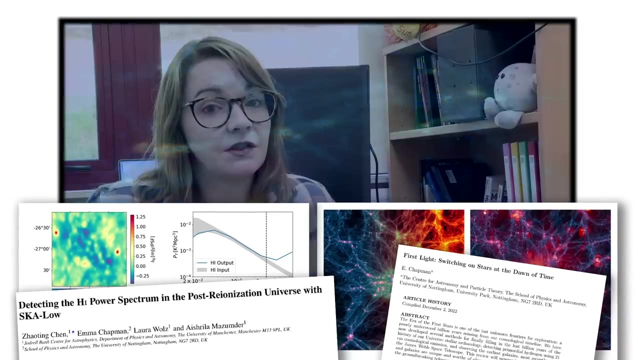 And you're right. People don't really care to plant a tree that they're never going to sit under, especially politicians. They care about a five year cycle, right, Let me ask you this: You're like a proper astronomer, Right? You do, you do, you know, you write papers, you do research on, you know early stars and things like that. 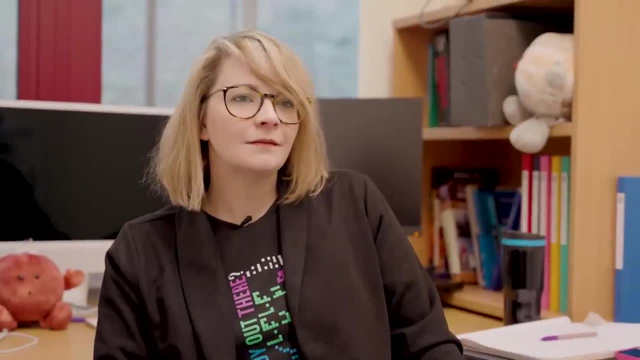 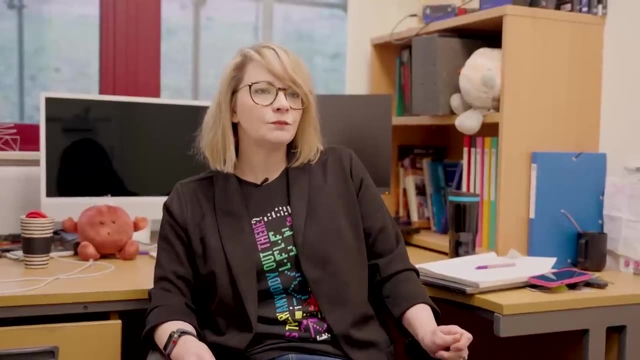 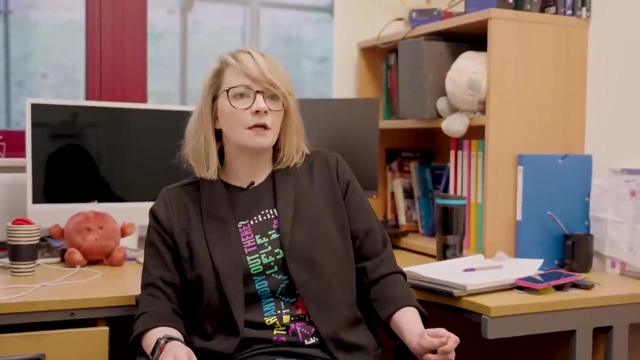 You also have this incredible passion and enthusiasm for SETI and the search for extraterrestrial life in the astronomical community. Are the people who also have this passion for SETI considered like a different class, or are they like? is that, are they like? Yeah, there's some eye rolling. 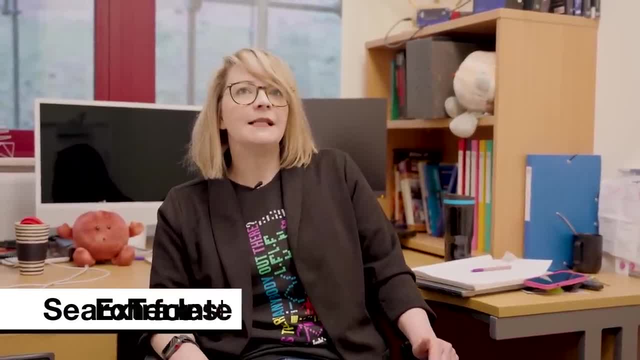 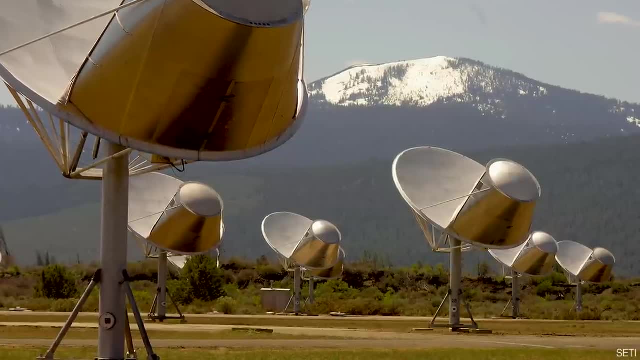 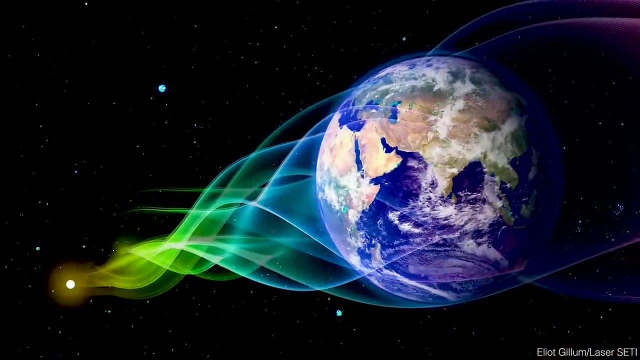 Yeah, I wasn't into SETI at all until about two years ago And I always considered it kind of a bit of the fringe area And it was only when I went research into it myself that I realized that actually they're really pushing the boundary of technology and science and the ability to filter signals and search for signals and the computing power they need of incredible stuff. 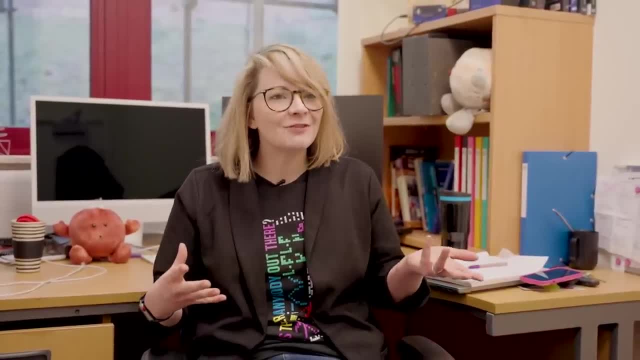 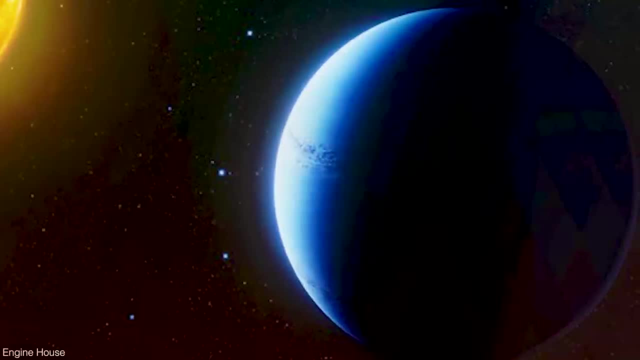 When I have mentioned to people that I am running a SETI project with the undergraduates, there's kind of like, oh, that's fun, It's not really. it's not really seen so seriously. I think the biosignature side. 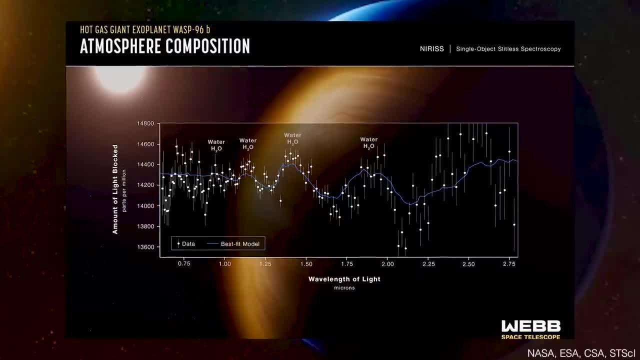 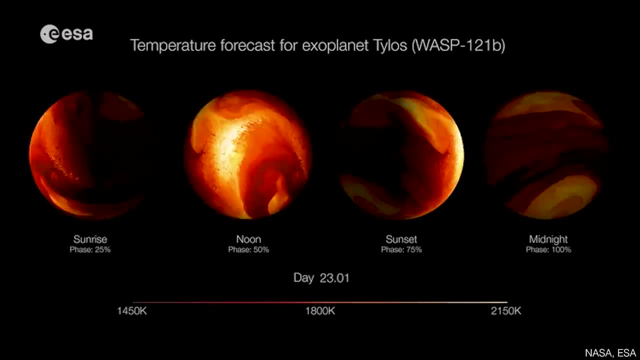 He's taken very seriously. So looking for biosignatures in exoplanet atmospheres. there's a fascinating area and really depressing area where they're looking for signs of climate change in exoplanet atmospheres. So they're like, hey, is any civilization destroyed themselves in a similar way to us? 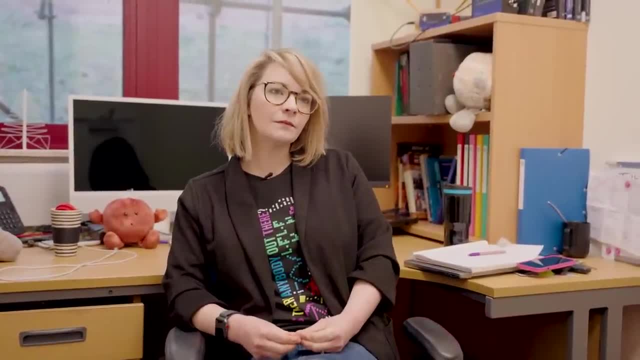 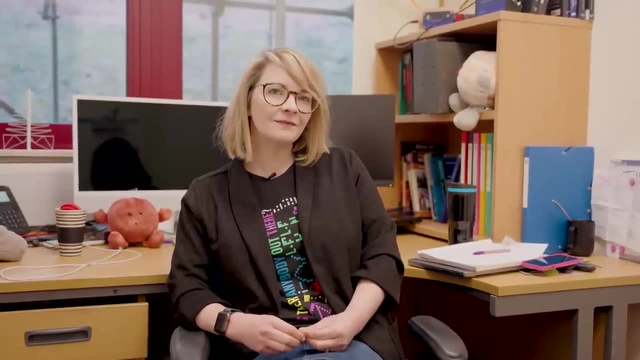 Because I speak to lots of astronomers and I know lots of astronomers and in much the same way, I think astronomers have to have to say, hey, it's not about like astrology and star science. right, You know that's, you've got it wrong. 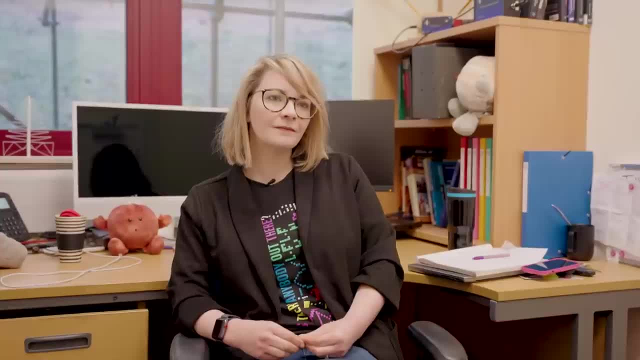 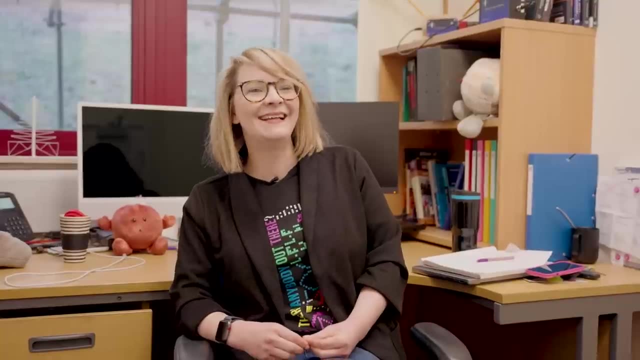 I also think sometimes they feel a little bit like: no, I'm not searching for aliens, It's not about aliens, That's not what astronomy is. But you are a fully fledged astronomer, but you are also really into searching for aliens and that sort of thing. 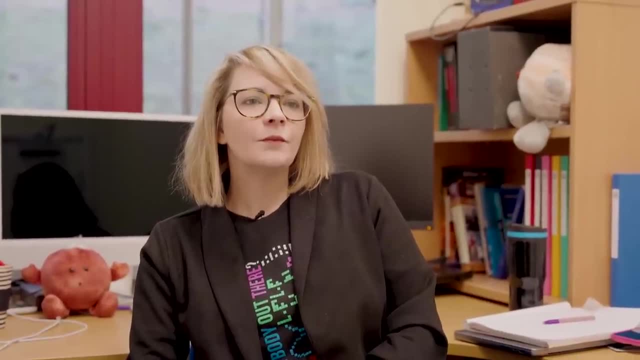 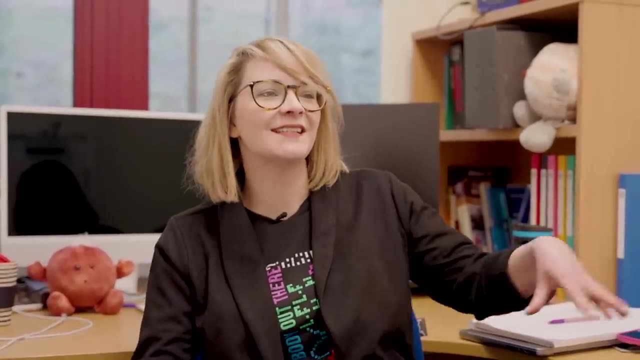 So I wonder: are you considered like a crazy auntie, or is there more acceptance within the community that this is legit? I think there's definitely a raised eyebrow at my kookiness when it comes to doing this as a as a side project. 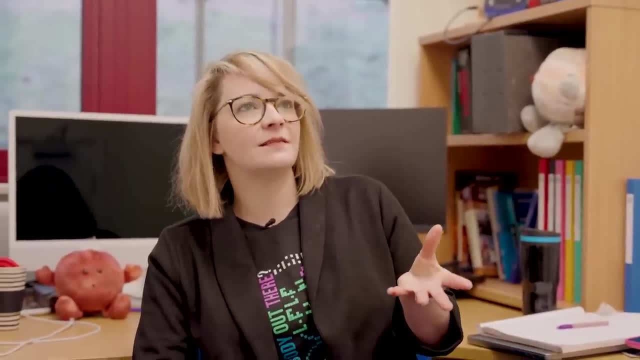 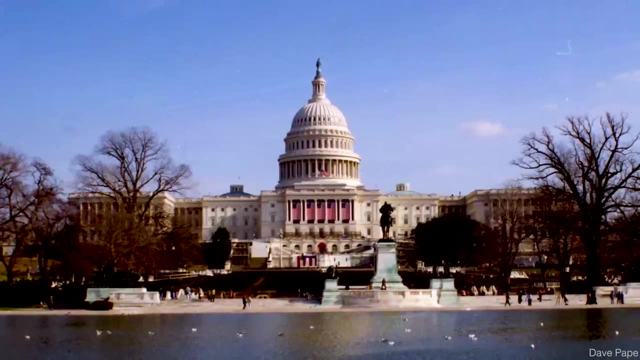 I fight very hard for the reputation to be to be repaired. This was considered a really Crucial scientific area in the 1970s and it was only when the politicians got involved and start saying we can't use our taxpayers money to search for aliens, and it became a political football. 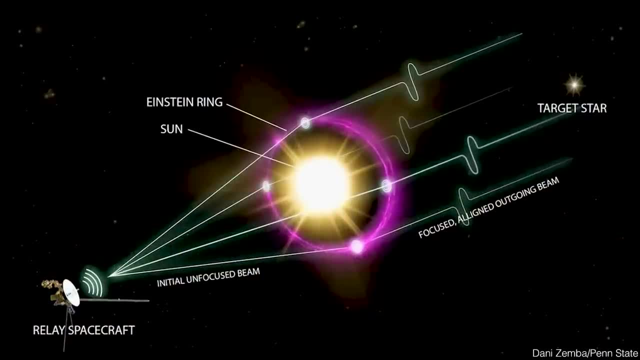 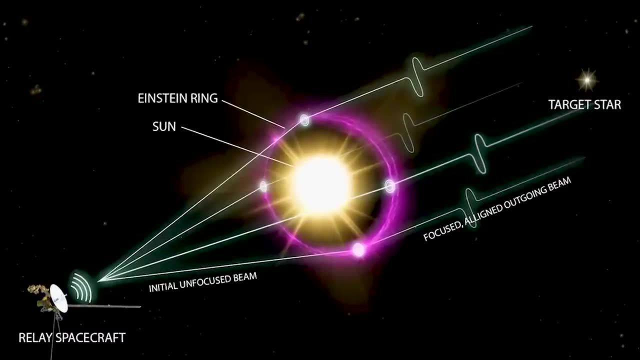 But, like I said, the science that I have to do. I'm looking at how a message is gravitationally lensed around the sun, for example. that's gravitational lensing. We've talked about that before. I'm looking at information loss and all sorts of techniques that actually I use in my search for the first star. 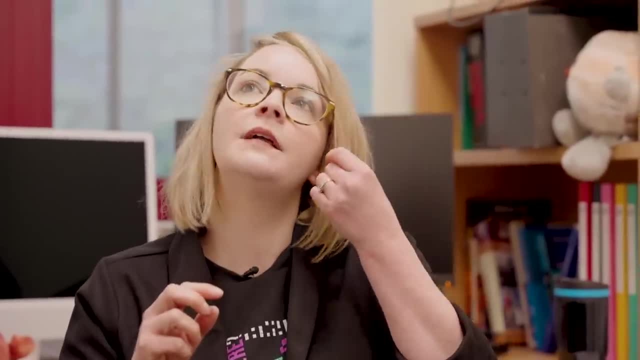 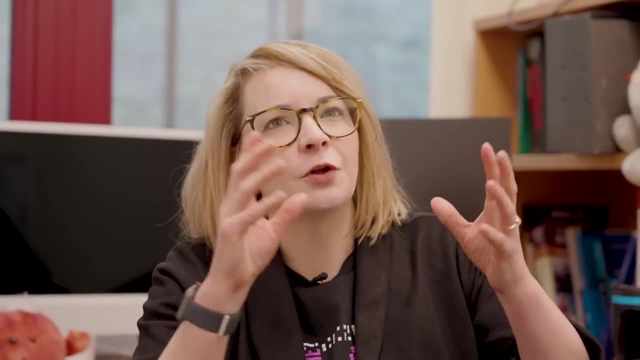 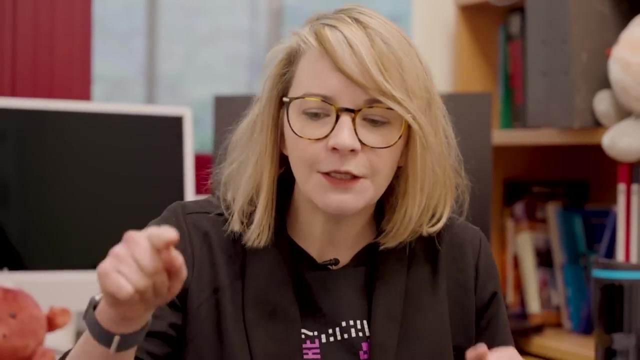 So this is it. I was in a control room of a radio telescope In California a few years ago and they were showing me this image of this drift signal where it turns off and on like the signal that we're looking for, and I saw them type in and they were like: oh yeah, we're just going to use this thing to search for signals like wait, I use that. 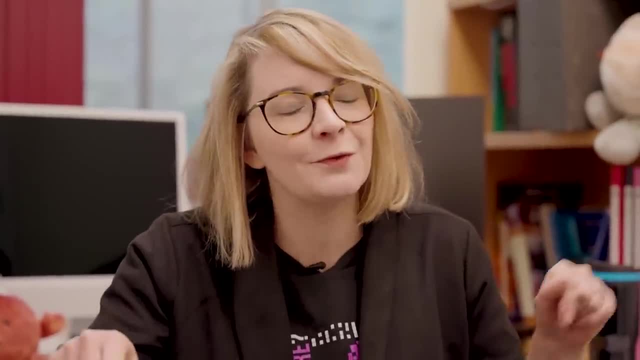 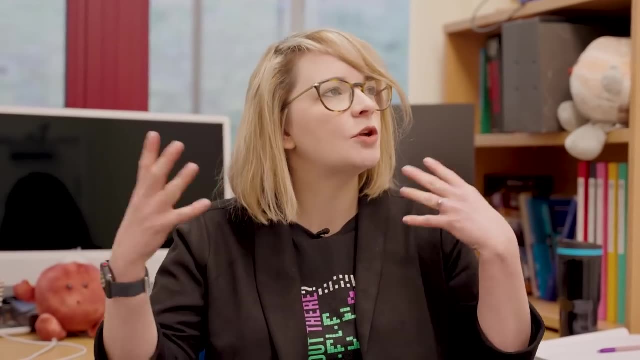 That was developed by my first stars team with Lofar, my radio telescope in the Netherlands, and I was like, hang on, I'm searching for a signal from the first stars. that's tiny, We don't know where it's coming from, what it's going to look like and it's got a load of rubbish on top of it. 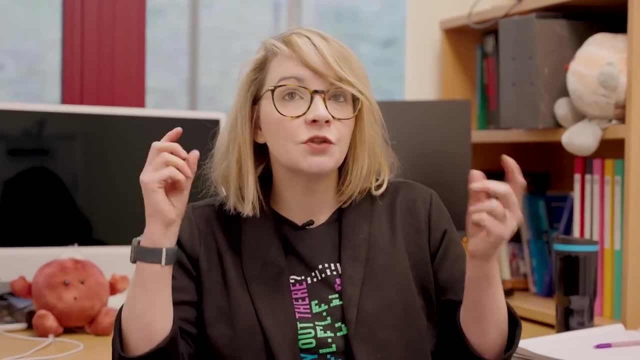 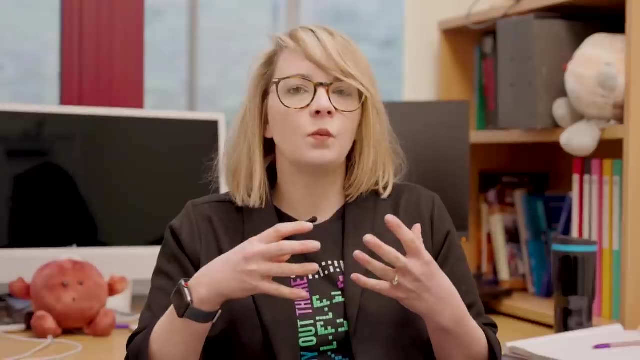 That's the same as searching for an alien signal, And so I just switched on. I was like I can just use these techniques And my answer to anybody who kind of raises an eyebrow I was like why not? Why wouldn't you do this while you're doing your other science? 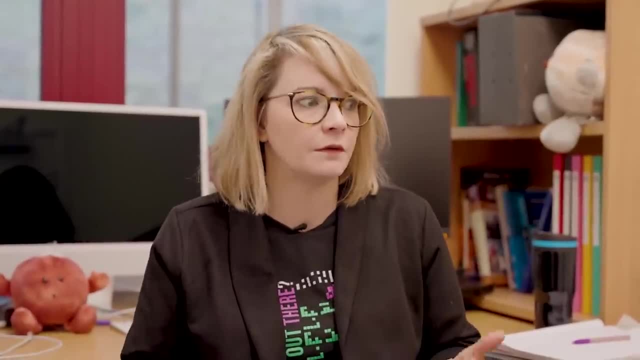 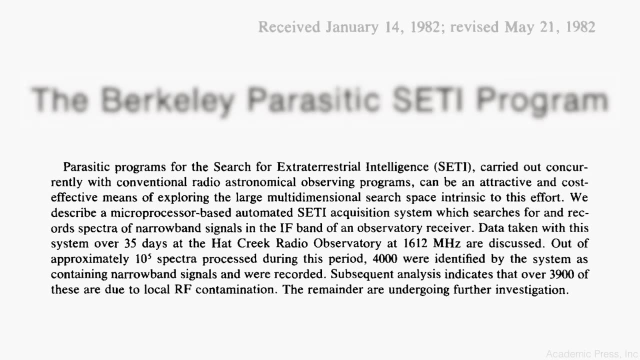 And that's what SETI has built itself up around. thanks to all of this, political funding cuts is they've become what was originally called like parasitic SETI, where they developed all this technology- that was kind of plug and play and they shipped it to Australia, to Lovell. 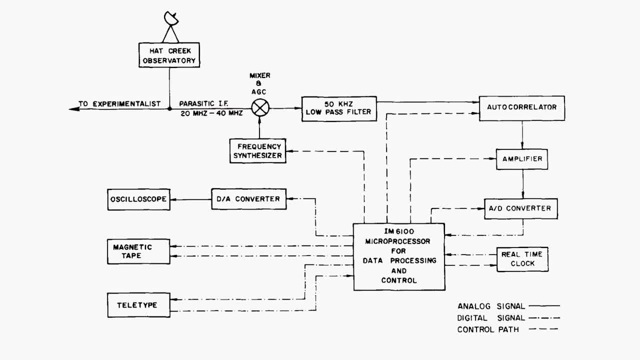 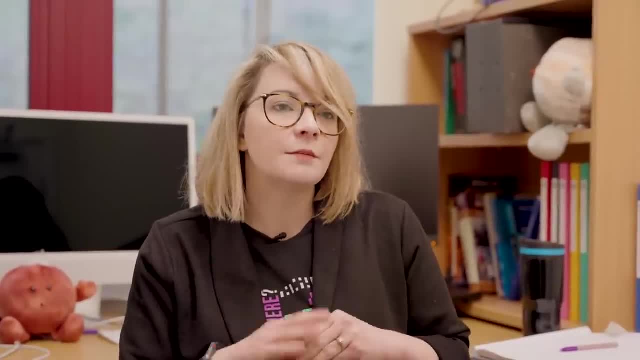 Manchester and they plugged it in And while they're searching for pulsars, they take that data and they also sift through it with their techniques And there's a lot of that going on. still, It's called Boutique SETI. now It's been rebranded. 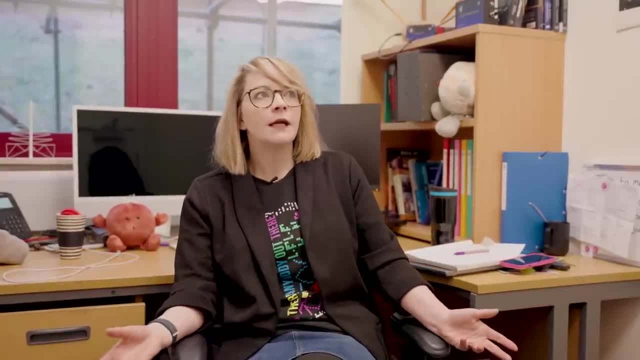 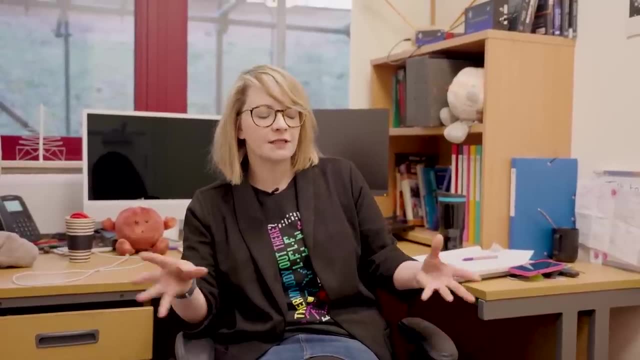 Why not? Why wouldn't you? And plus, you know we're not actually taking taxpayer dollars to do this anymore because of all of these cuts. They were so clever and they created their own charities and their own institutes, And it's basically funded by billionaires with too much money. 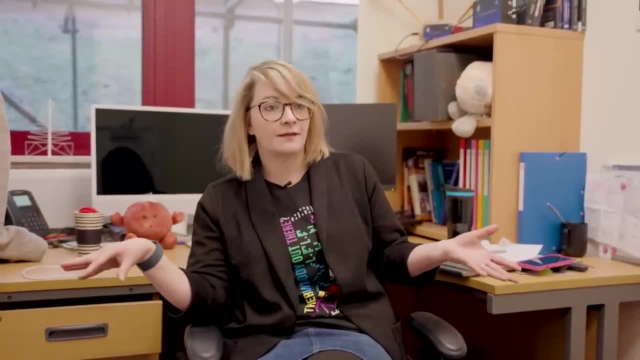 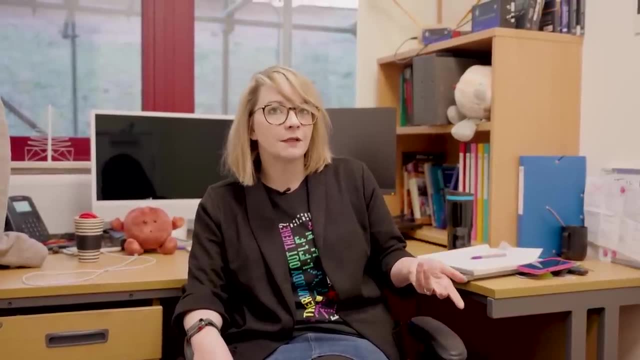 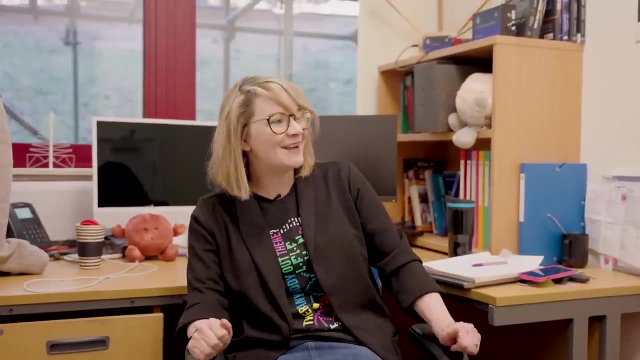 And a win. They have the will to put their name on everything, including First Contact, and they give. they give hundreds of millions of dollars. Steven Spielberg has given $100,000 because he said it's about time that he invested in some science, fact which I thought was beautiful. 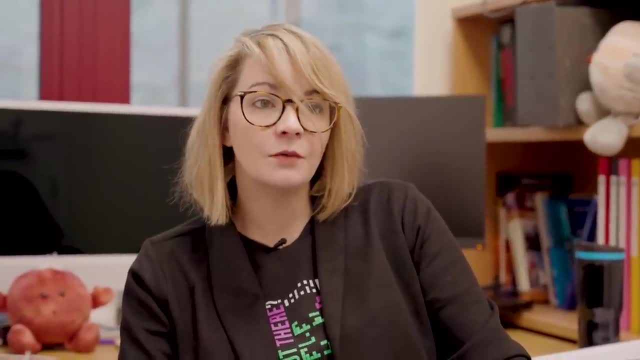 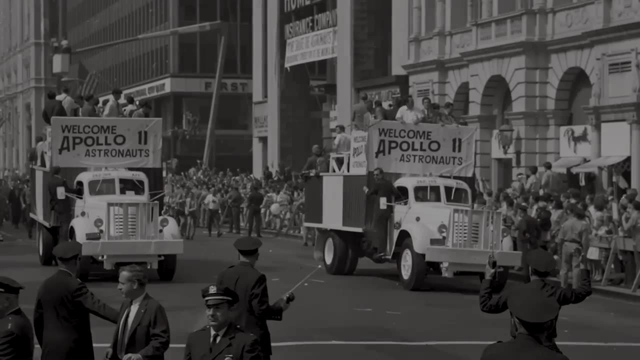 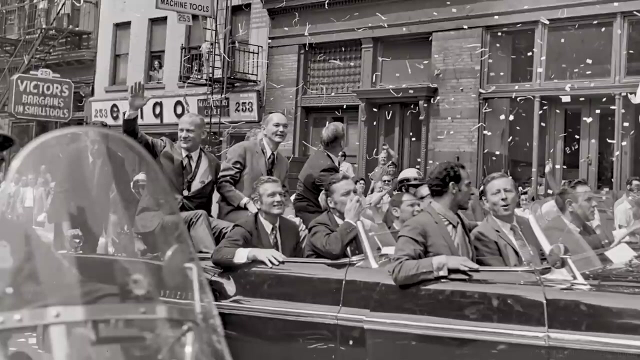 Yeah, but it's mostly Microsoft, Google, Hewlett-Packard- all the big names fund this now, and just random Russian billionaires that you'll have never heard of. Humans love stories, Humans love heroes, They love like the first person to put their footprint on the moon, and things like that. 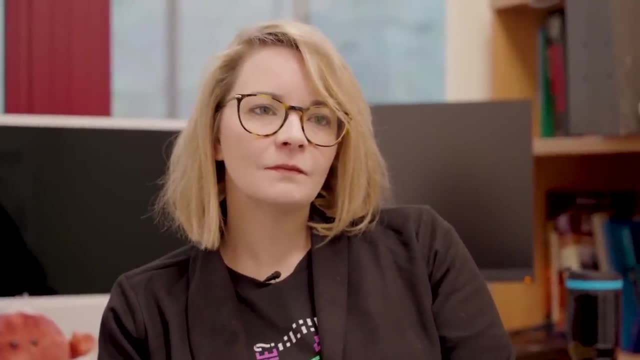 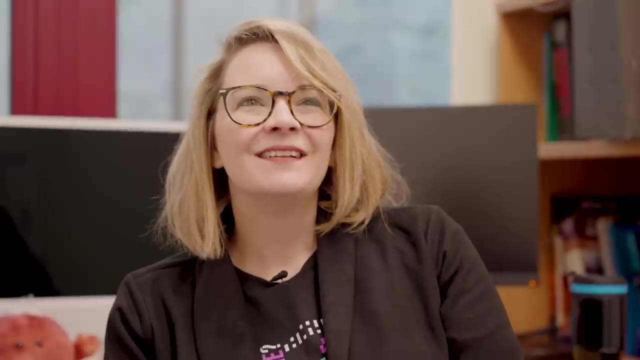 Will First Contact have a hero? Will there be a person who happens to be on call at the time, like that moment when you know Jodie Foster? Will there be a moment, Is it like that anymore? Or will there be a first person who heard it? 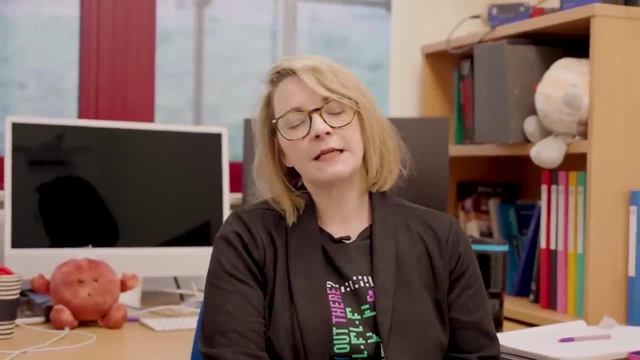 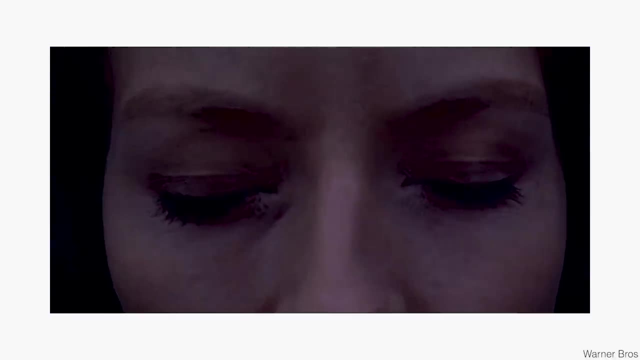 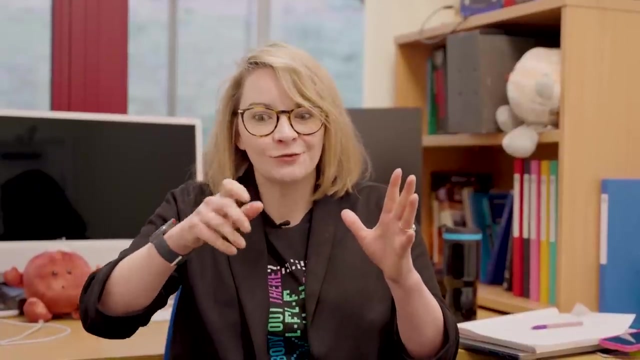 I think there will No. Okay, so very unlikely. because when Jodie Foster was looking in Contact for anybody that doesn't know that film, so much fun. Also a book- Yeah, she was listening and heard it, but that was kind of you imagine your old radio. if you had one, you tuned it into Radio 4 and you listened to Radio 4.. 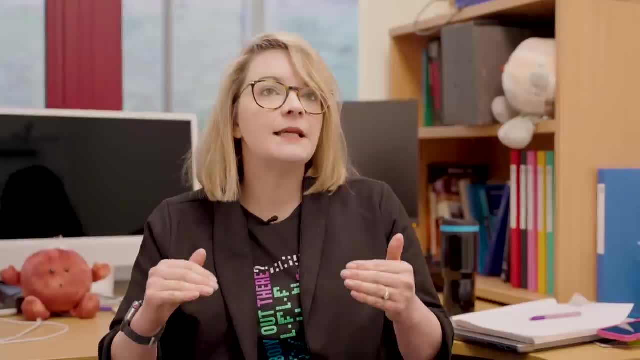 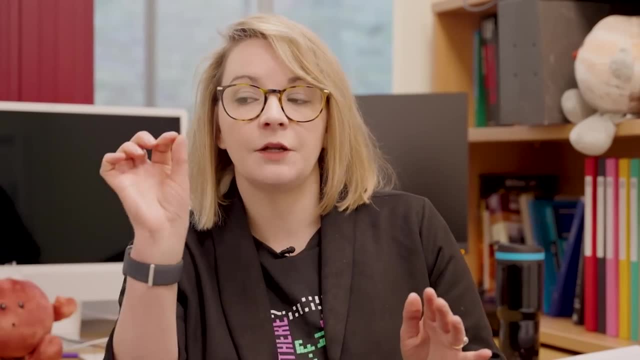 That's all we used to be able to do. Now SETI is about having the most powerful servers in the world and they scan every single radio channel in incredibly fine detail over all of the bandwidth at the same time. A human doesn't listen to that. 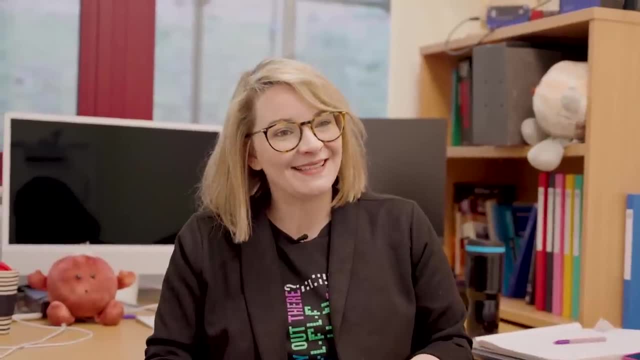 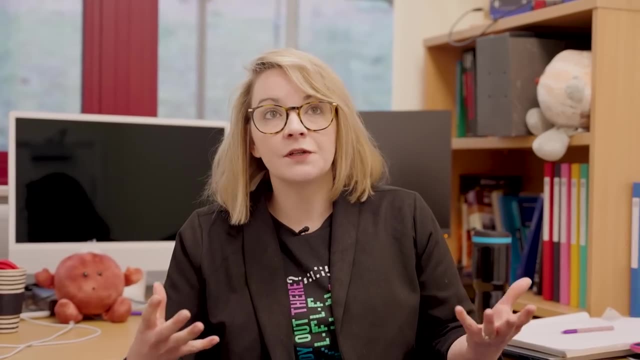 It's this algorithm. Will there be the first people that get that message, That automatic message? Yes, I think Jill Tata, if it is within her lifetime, and I'm not saying anything about her age there, because Contact could very easily be in 102 years. 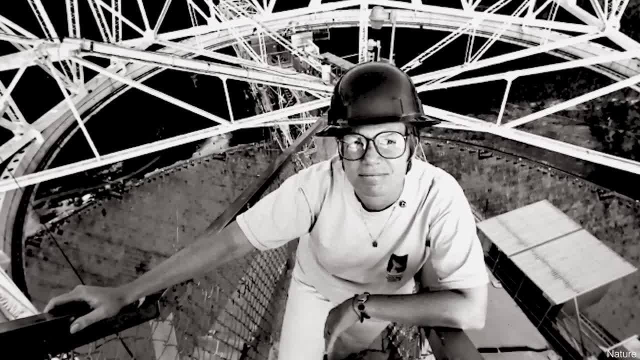 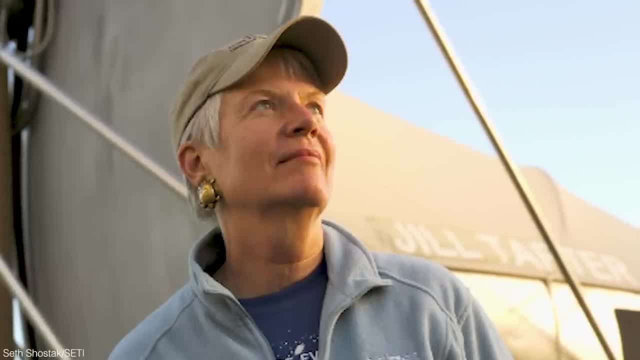 Jill Tata was one of the people that really kept SETI going during the funding cuts. She's incredible history. If it's her dedicated array that she helped build, she learned to fly so she could get to this remote location. I think she'd be the hero. 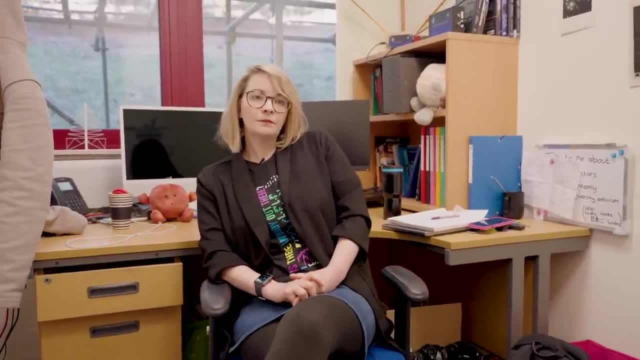 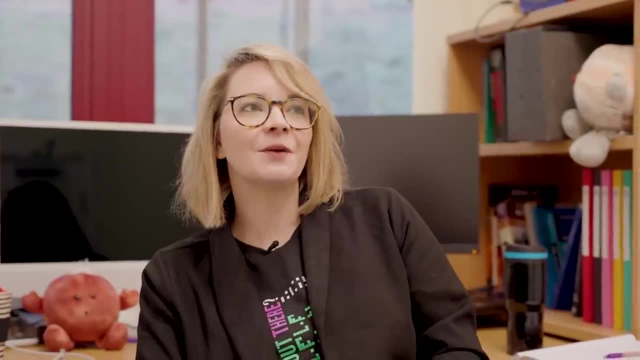 You can't talk about the search for alien life without this thing that lots of people have heard of But might not understand, called the Drake Equation. Can you tell me what the Drake Equation is? The Drake Equation? I'm going to quote Jill Tata and say it's an incredible way of organizing our ignorance. 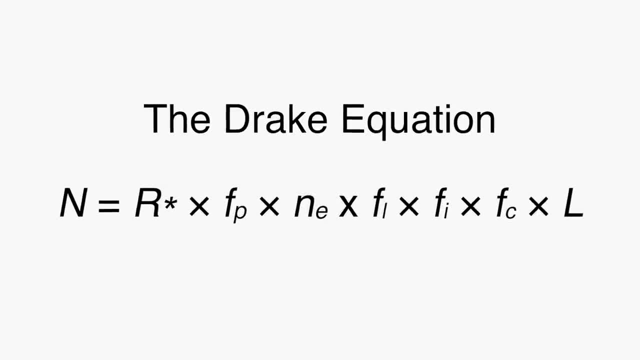 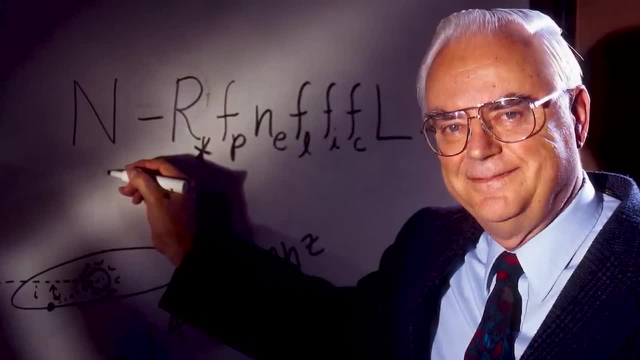 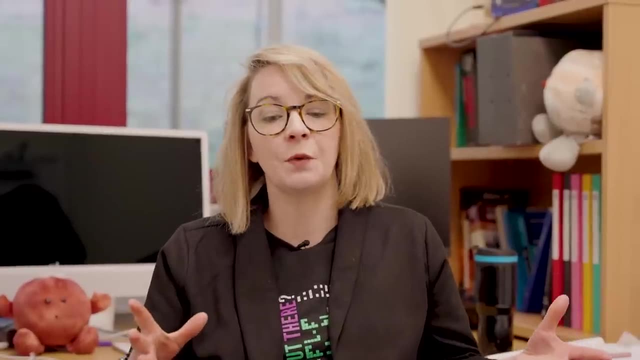 It is a series of symbols very apt for this channel, which was written on a chalkboard in 1961 by Frank Drake, at the first ever meeting of minds on how do we search for extraterrestrial intelligence, And he brought together all the people interested in the world, which he said was about 10.. 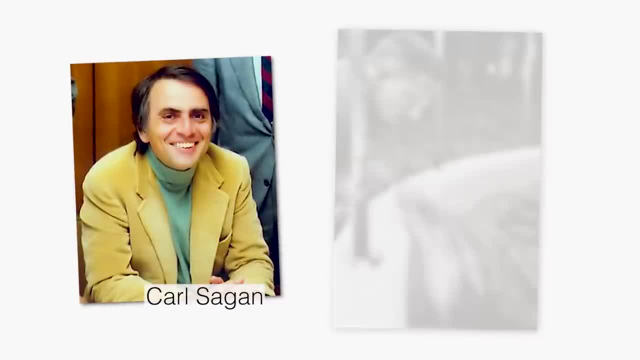 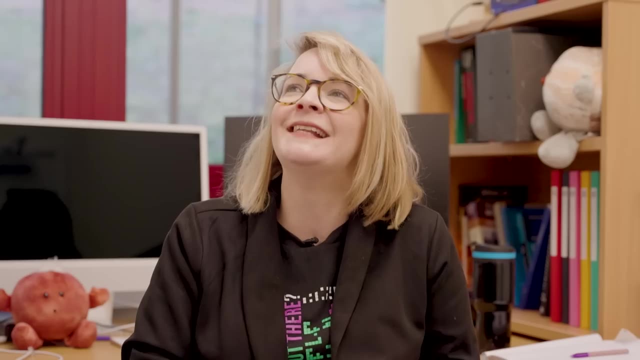 He included people like Carl Sagan, a science communicator, but also someone who was researching how to talk to dolphins And he was taking LSD and going in and talking to dolphins. But at the time people thought he was serious, because we want to know: how do you communicate? 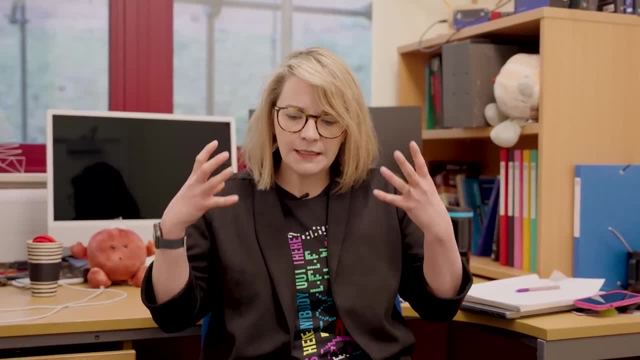 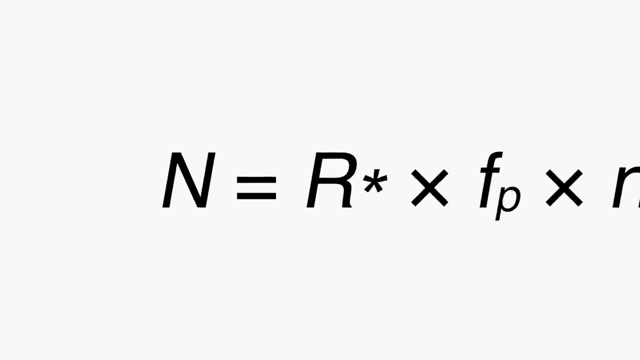 So it's all these different meeting of minds. It was like: all right, what do we need to know to contact aliens? So he wrote this equation on the board: On the left-hand side is n, And that is the number of intelligent extraterrestrials. 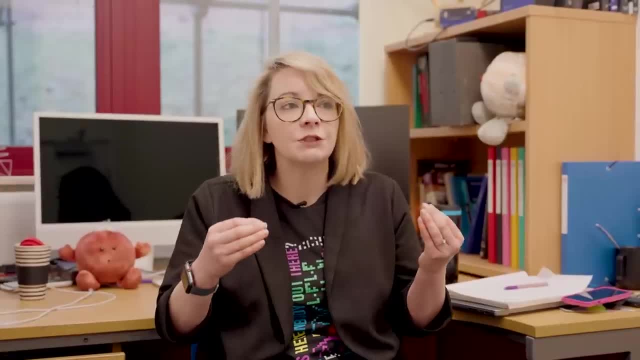 It's the number of aliens that we can contact. It's the number of aliens that we can contact, special civilizations that we can contact, and all of this is a bit tongue-in-cheek. it's meant to be an agenda for a conference. people get all excited like let's calculate every bit. it's not meant to. 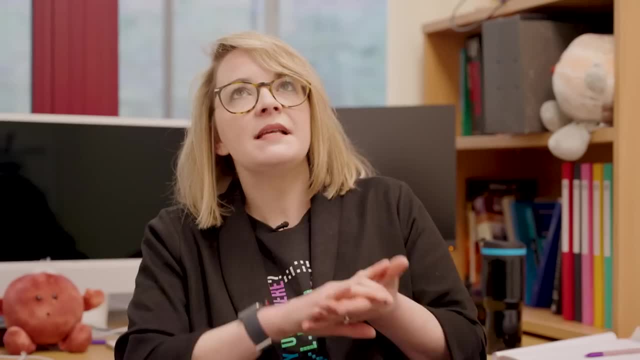 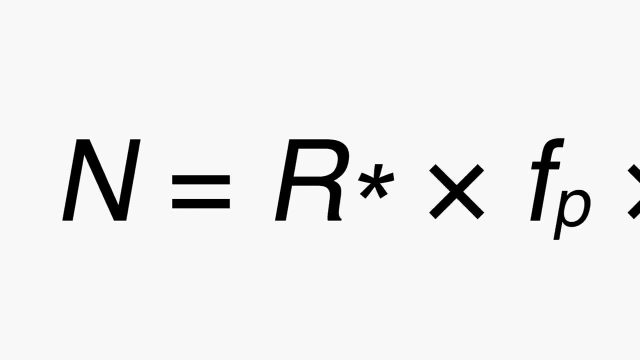 be that it's meant to be this way of thinking, so n is it possible? then we go on to the right hand side and we're like: right, what do we need to know? first of all, how many stars are there? how many stars are there formed per year? and we're talking about, you know, a star formation rate, where you've 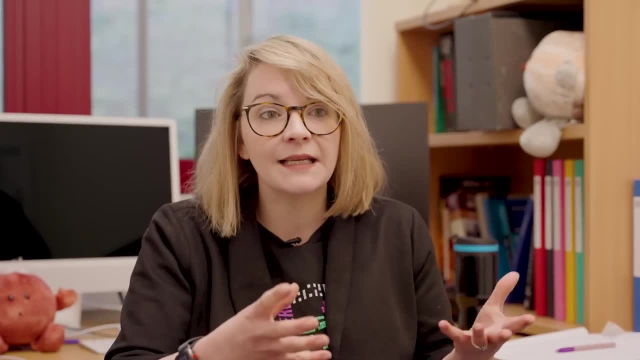 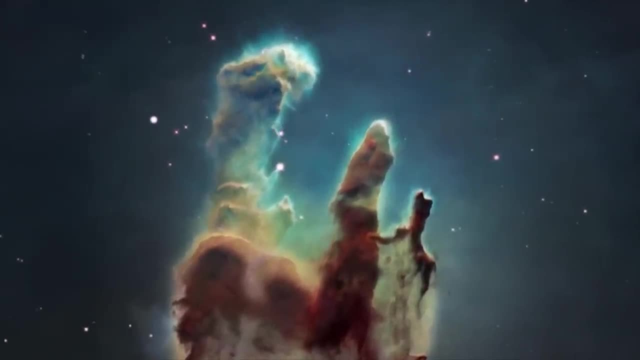 got maybe 10 stars a year formed in a particular in the milky way. it's very low. i'm always surprised by that, um, but you kind of need a star to create planets, to create life. so how many stars then we're going to filter? and i always think of this as kind of like when you're searching for clothes. 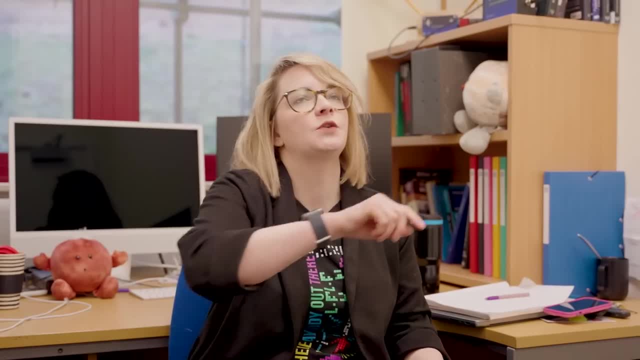 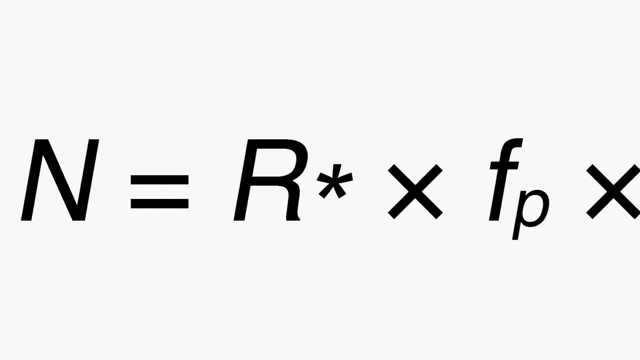 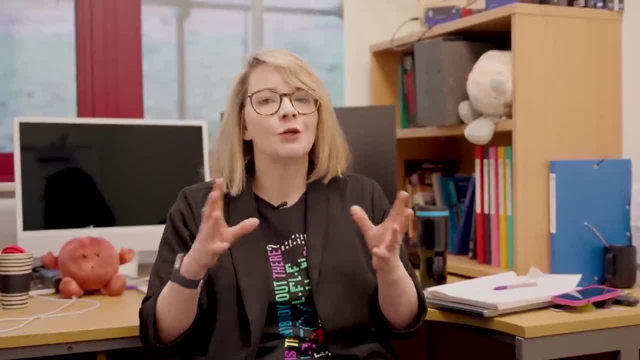 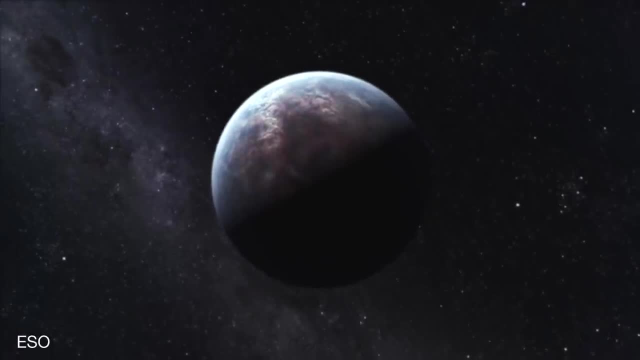 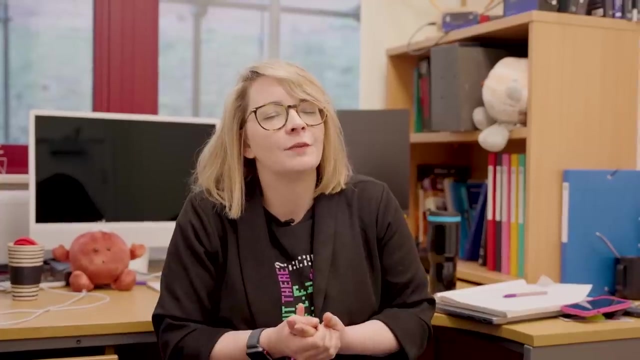 form a planet. since frank drake's- frank drake's time we've done so much research on exoplanets, so we're quite happy that that's. that's really high, it's, it's, it's one. basically all stars can form planets like. there's very, very few that that will blow themselves up so quickly they can't form. 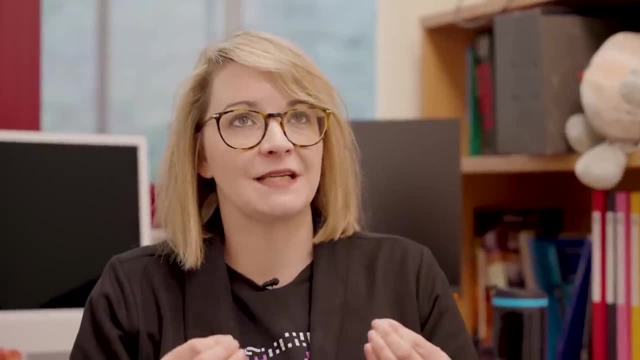 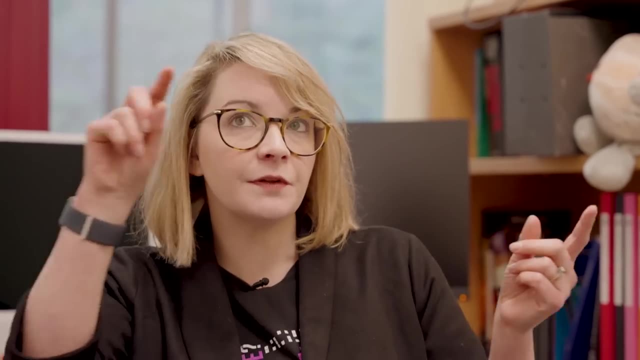 planets, so fraction of those one. it's really important not to get bogged down in the exact numbers here. it's more like it's a philosophy. yeah, are there enough for us to keep searching on this filter on our website? yeah, there's still a whole load of stuff in here, so let's keep looking. 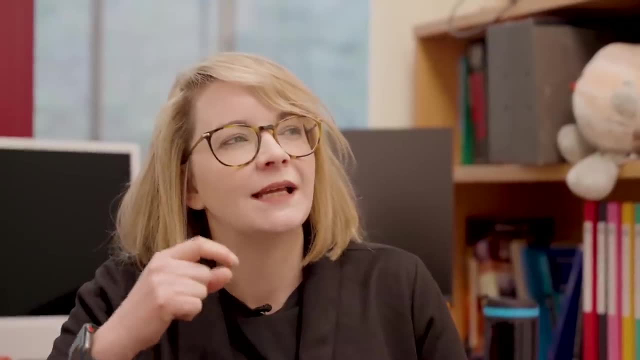 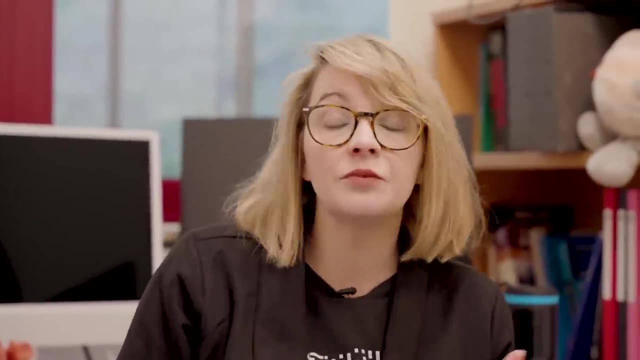 so that's what we're doing here. we're slowly filtering in every stage, saying: is it worth looking? so are you looking for? basically, you're looking for a deal breaker. yeah, we are, we're looking for a deal breaker. the deal breaker isn't the number of stars, we're fine the deal breaker. 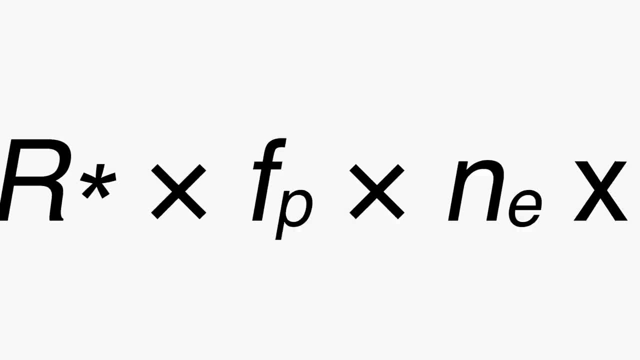 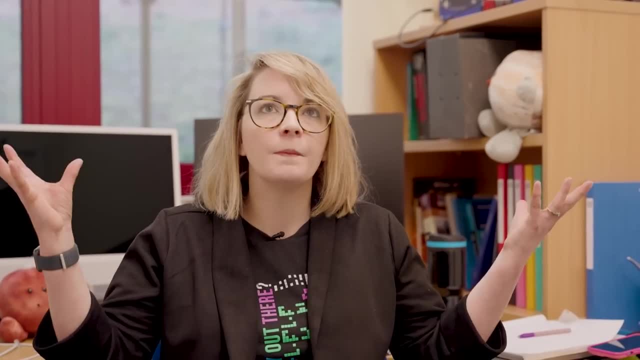 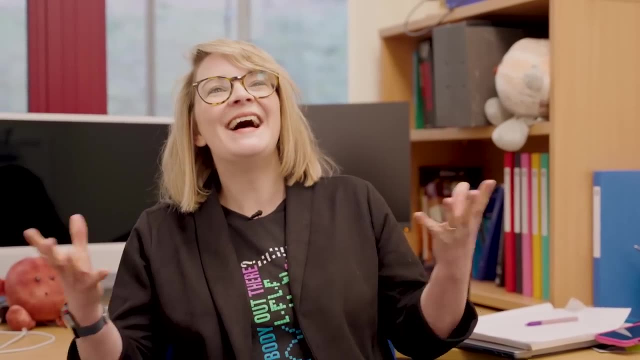 is not the number of planets, we're good, then we're going to go on to how many of these planets actually form an ecosystem. so have an atmosphere that can protect them from the sun's rays, for example, um, and create an atmosphere that's that's, that's breathable if those people have lungs, um, and 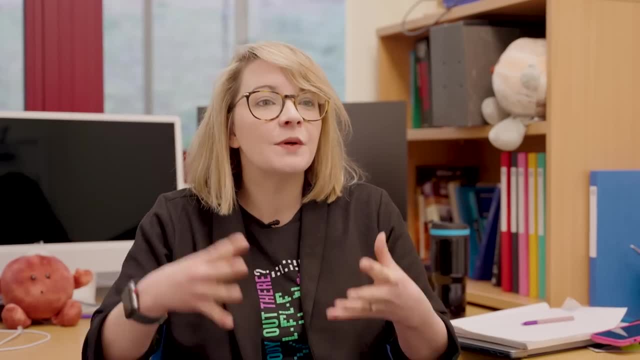 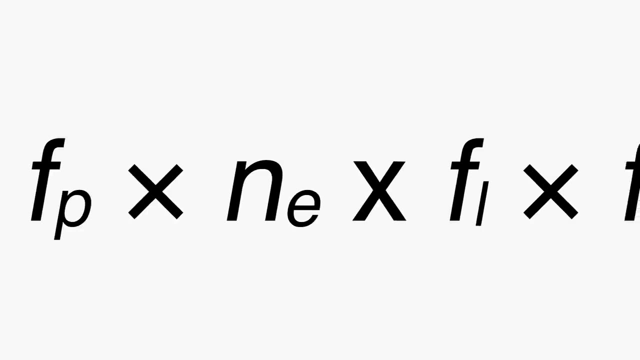 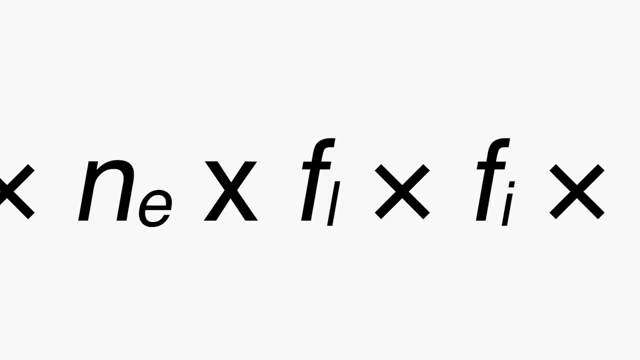 that's you again. 50 ish. you know we're talking about a really large 30 to 50 kind of range of planets that might form this kind of atmosphere. but then how many of those can form life again? we're kind of like just balancing numbers here. but let's go 50 again. you know, now we get to the 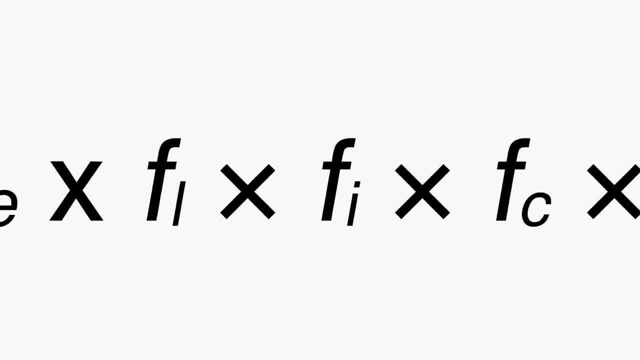 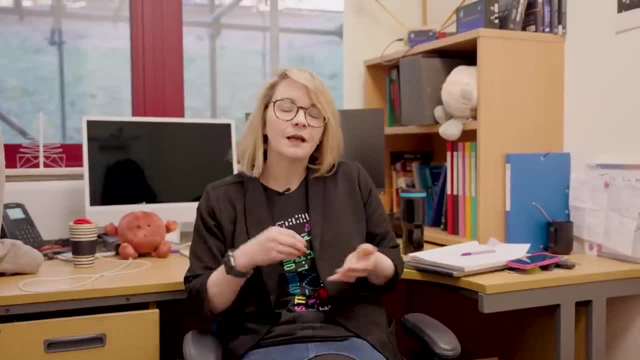 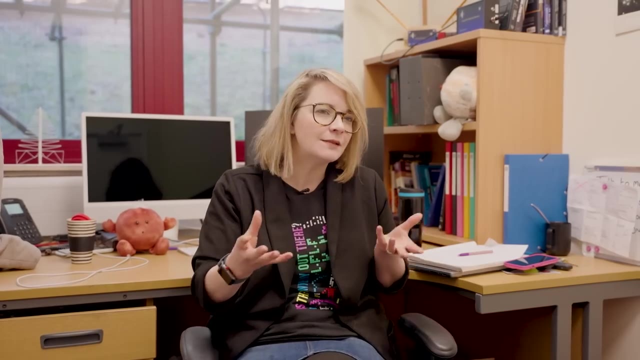 deal breakers. how many of those planets, what fraction of those, can form intelligent life? this is where we just don't have a clue. we've got a sample of one at the minute, but is there really any barrier to evolving intelligent life once you've started evolving life? not really, it's. 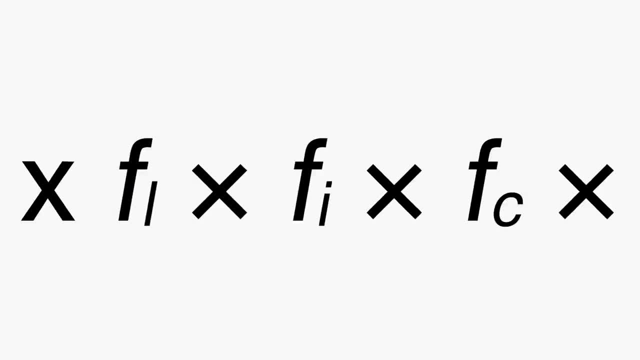 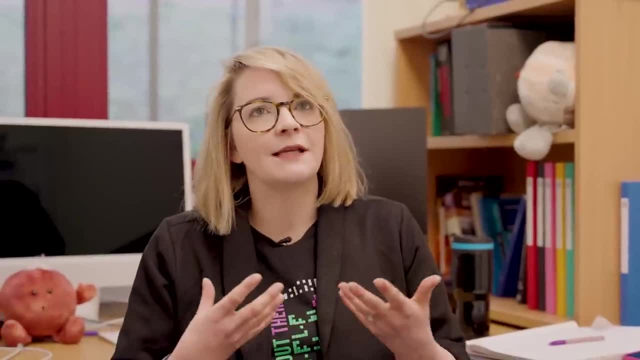 more about time, isn't it? so let's keep going. let's keep going on to that. now we've got intelligent life. what fraction of those can create a way of contact? how many of those develop, let's say, a radio telescope? so you're going to want an atmosphere that lets radio waves in. uh, you're. 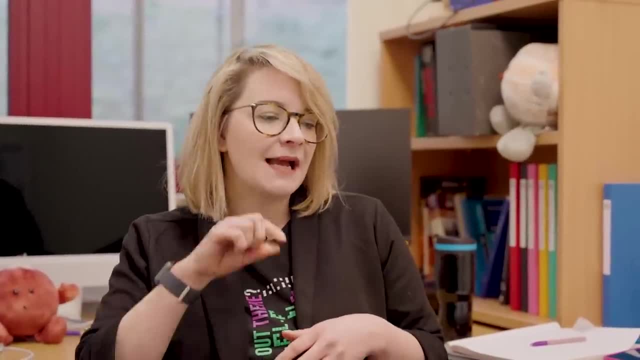 going to want a curious civilization. um, at what rate can you create a way of contact with a mission? so what fraction of this can develop the information that's going to be used to create a truly intelligent life? so it's so easy to understand and it's very difficult, but it's. 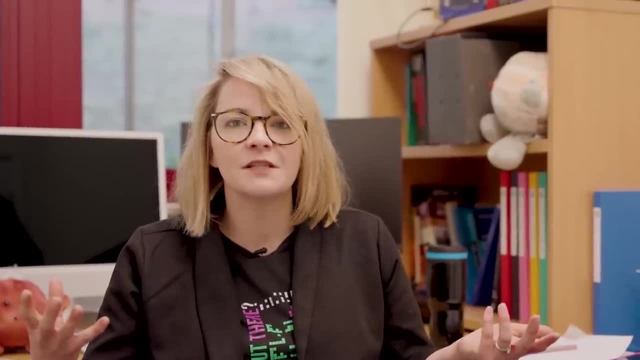 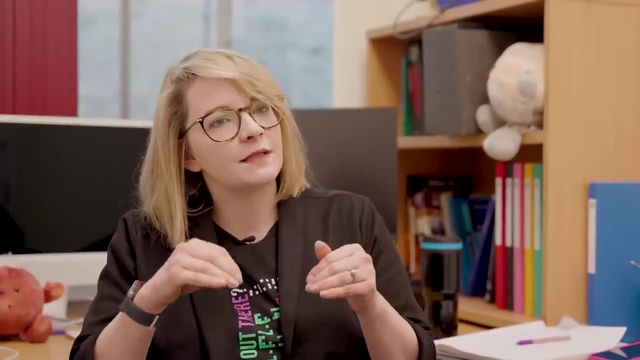 very difficult to government. you know it's. it's a very difficult thing to do, but at one point somebody added a symbol to this equation that was like f, sp, which was the fraction of stupid politicians that you had on the planet. because even if you do develop these radio dishes, the 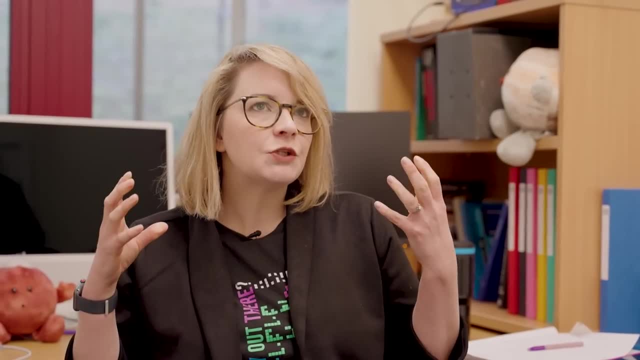 politicians can pull the funding at any point, and this is- this is a bit of a deal-baker for me at this point. so the fraction that can create a communicative device and then sustain it takes a lot of power to to send out a message, and you don't know which planet. to you, I think. but um, I mean, it's a. 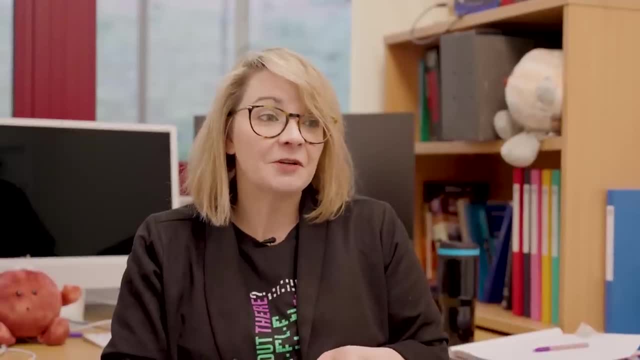 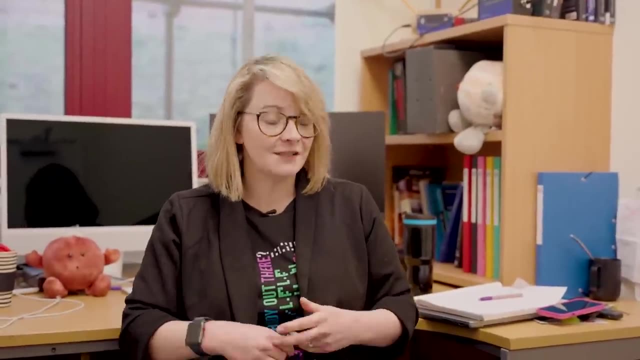 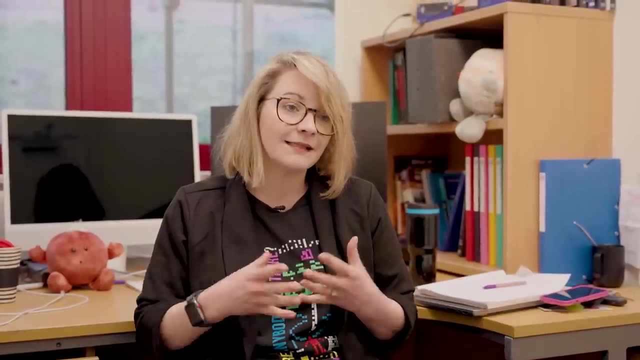 to point at um. so you're going to want a civilization that has huge energy budget as well. but we've done it. we've done it. we have sent a message in the 1970s that this one here, um, and we have been sending messages out since radio and tv began. this is actually called the. 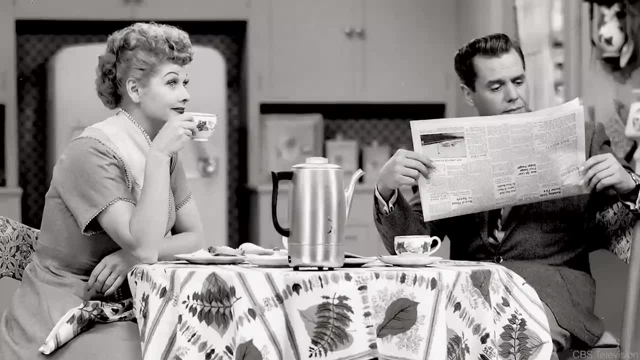 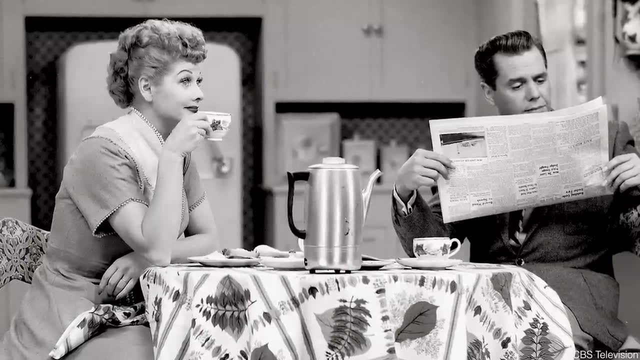 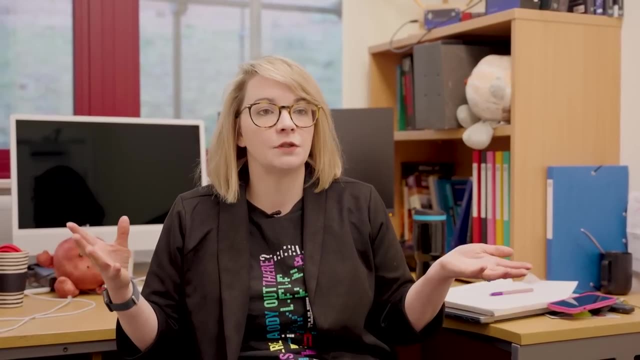 i love lucy. radius um because i love lucy- was the first mass produced sitcom where everybody was listening and it went everywhere on every radio um tv broadcast and so that radius is running at about 70 light years, so if you're within 70 light years of earth you can probably tune into. i love. 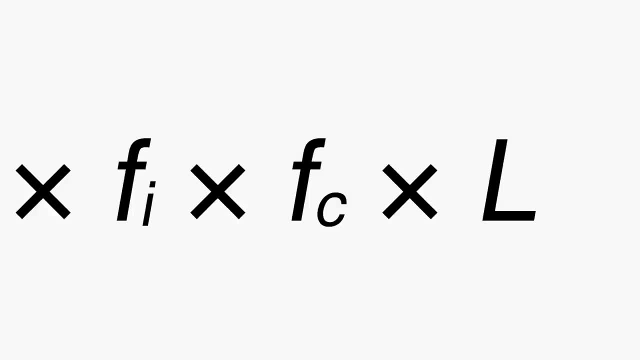 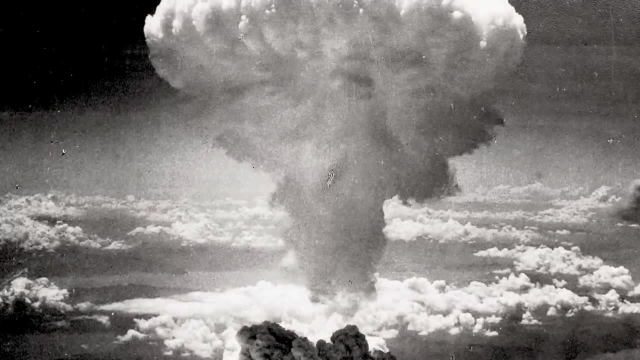 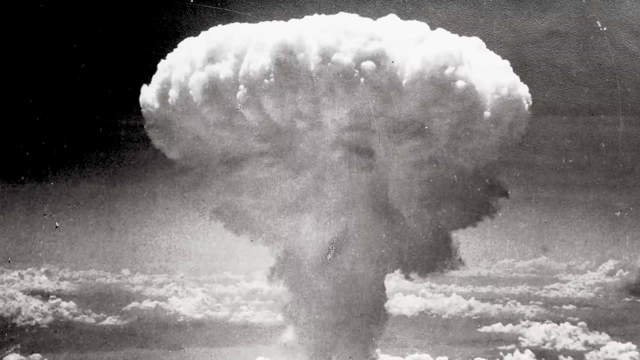 lucy, and know we're here, um, though it would be quite faint. last one, and this is the bomber. the last part of this drake equation is l nice capital. l carl sagan represented it with a mushroom cloud when he did this, because this is how long a civilization can last. you can do. 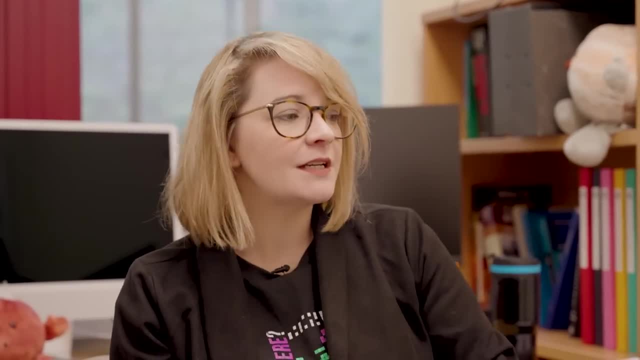 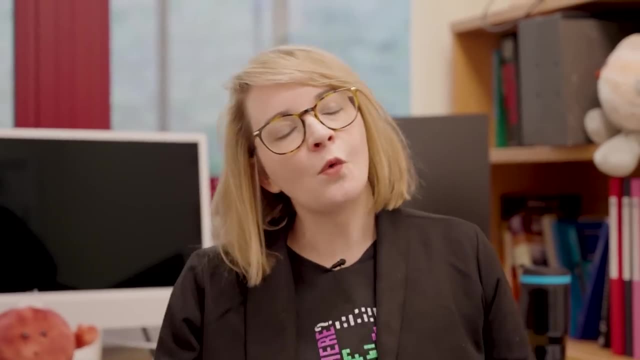 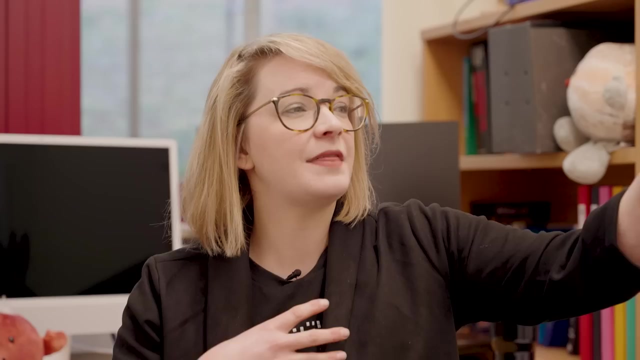 all of this. you can create life, you can create a radio, you can convince the darn politicians to keep funding you. but if there is so much war that your civilization blows itself up before, you can communicate that out to the right planet. and if that civilization, aka us um, blows itself up before, 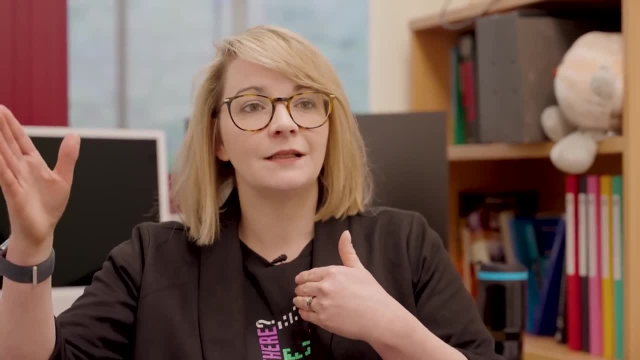 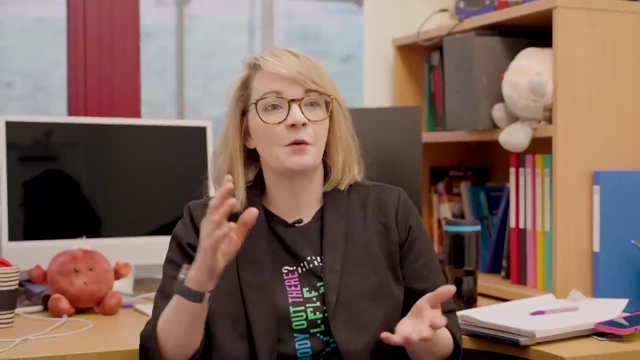 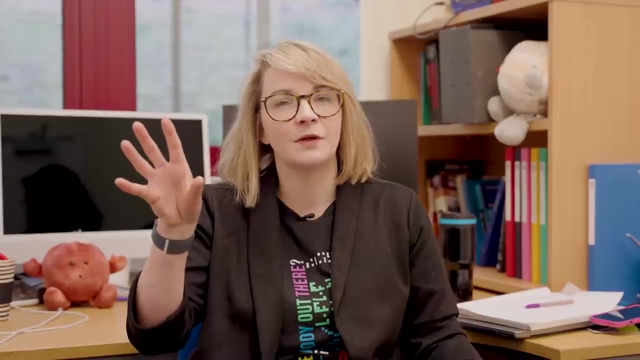 we have managed to listen to the right place, then it's all wasted. and so this equation condenses down to n equals l. so i'm going to do that wonderful spherical cow thing of let's just make all of those things go away, all those factors. we're kind of convinced what matters is: can we survive long? 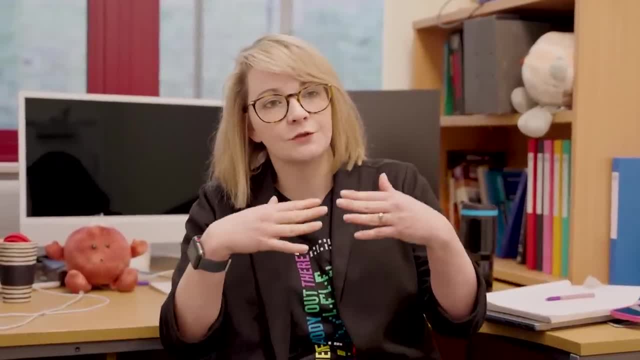 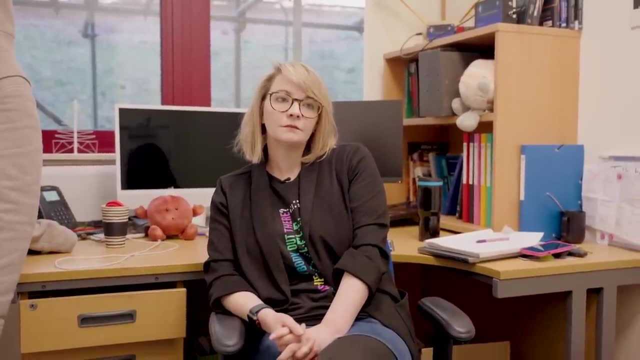 enough, and can they survive long enough that our communications cross over? that only matters if we want to communicate with them like they've only got to exist for 30 seconds and send the message for them to have existed. yep, so l only matters if we want to talk to them. yes, doesn't that like it? 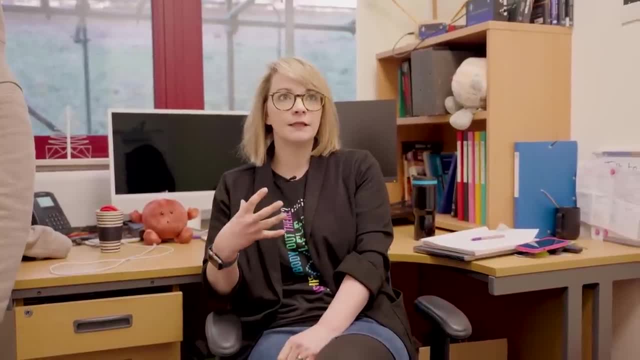 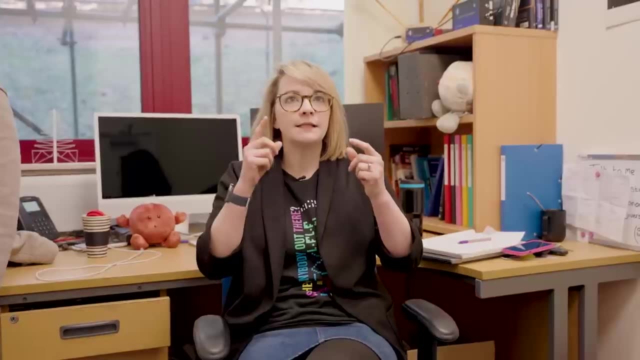 doesn't matter, or if we want to have a really good chance of listening to them, because, yes, they might have only existed for 30 seconds to to send this message, but we might have only listened to that planet at the wrong time, so we don't actually have the capability of listening to every single. 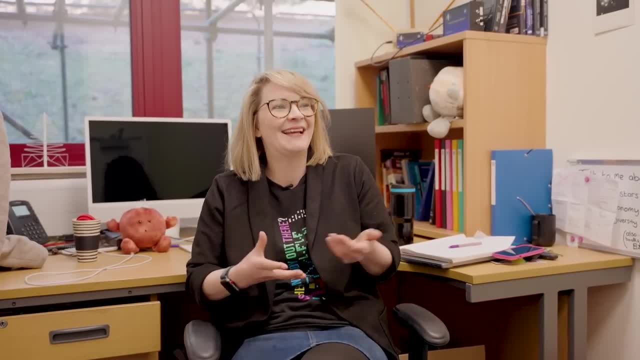 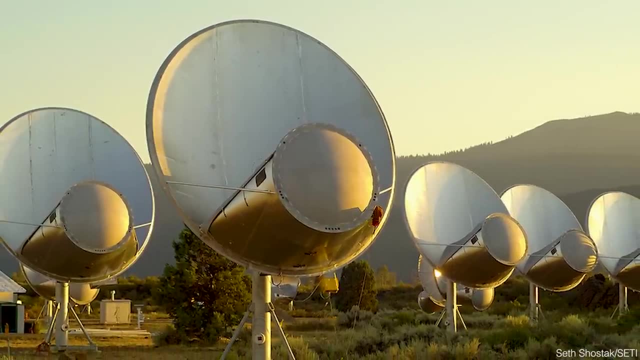 exoplanet. that's in this like we have a catalogue of habitable exoplanets, and what this allen telescope array does is it turns all of its dishes and it listens for five minutes and then it goes to the next one for five minutes and it repeats that catalogue of 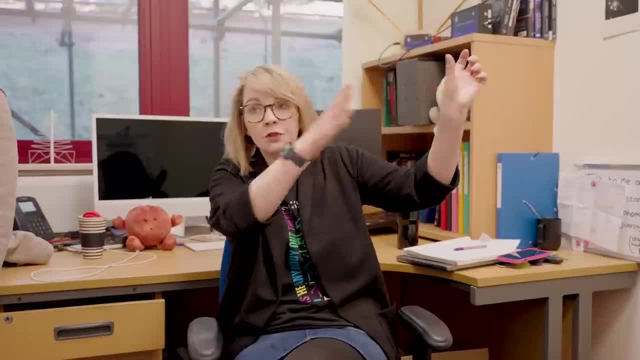 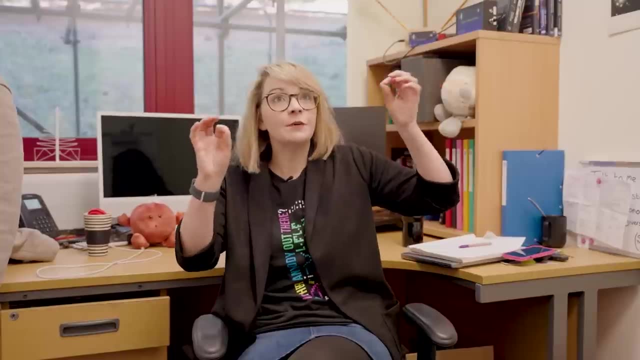 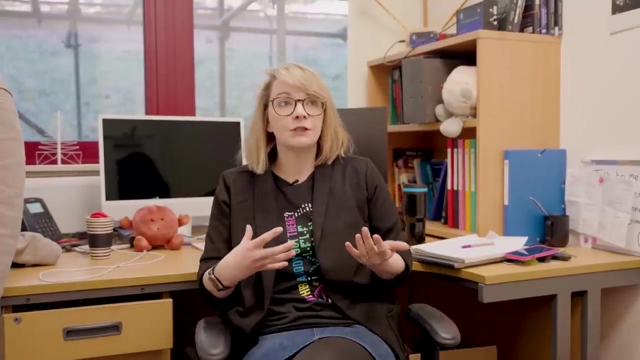 of 200 or something, and it's going to do that for hundreds of years. if we've just looked away, we're an et phone home. you know we've missed it, and and so, actually, when you're thinking about this, in terms of the probabilities of us being able to make contact, this civilization has to. 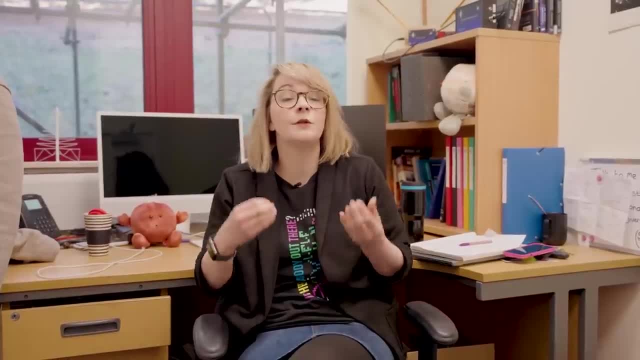 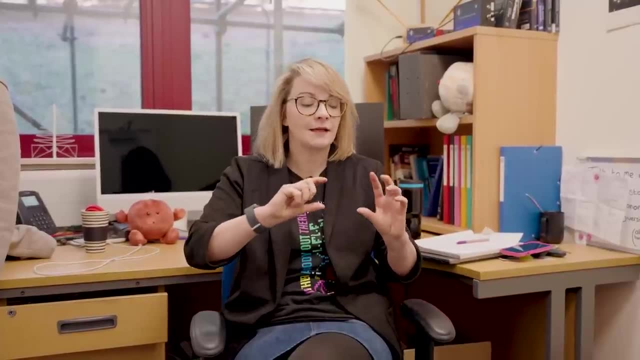 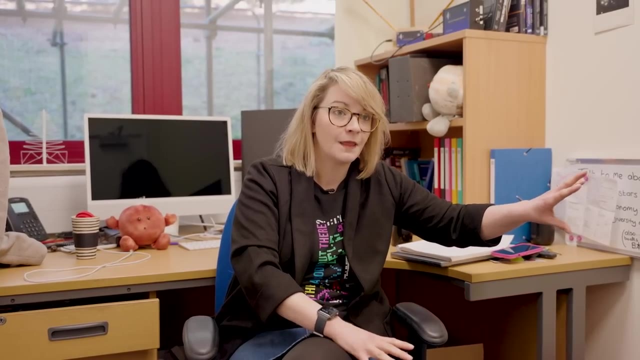 have been lasting a really long time and sending a really long time. but you're right, you can stop caring at any point in this- and the SETI Institute- it has hundreds of scientists on each of those things that only care if it develops life of any form, only care if they've got bio signature or you. 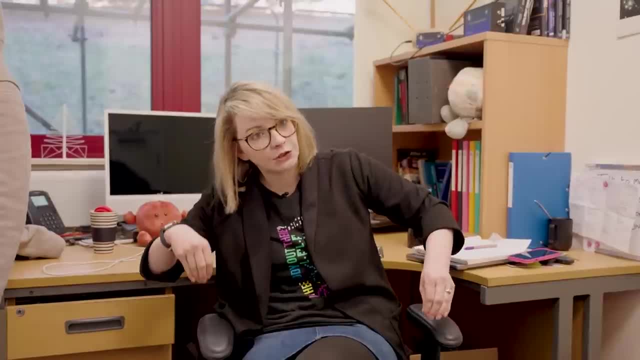 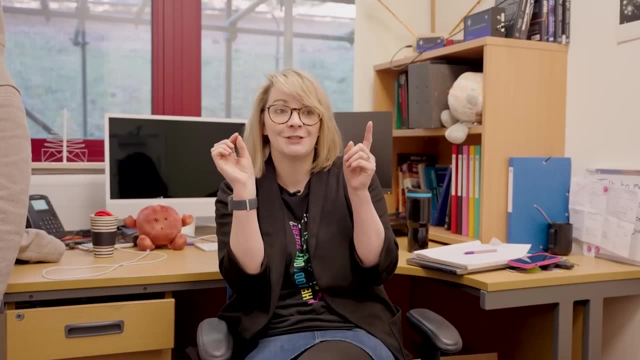 know, and it's only kind of the people that are really searching for extraterrestrial intelligence. this is the cleat that the SDI are the key right. it's the search and the intelligence and that's when you need the whole equation. so n in the Drake equation, as you've explained, the 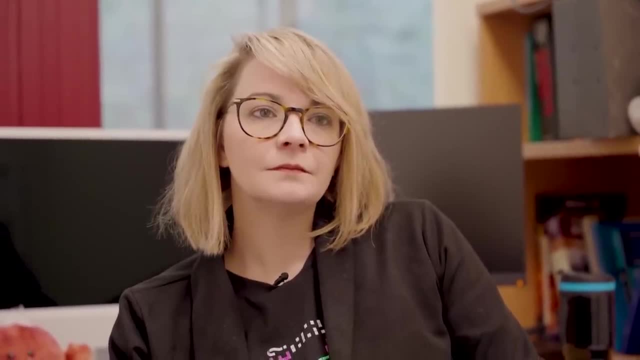 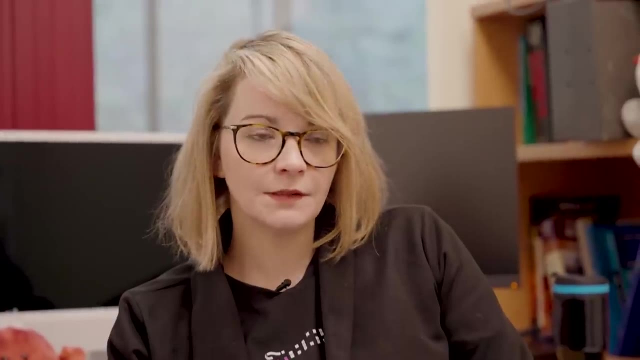 Drake equation with L included, isn't the number of civilizations that are out there, it's the number of civilizations out there that we're going to get to hear. it's the contactable civilization. contactable here, listen, listen to a bull. yeah, it was Frank Drake's number plate until he died was. 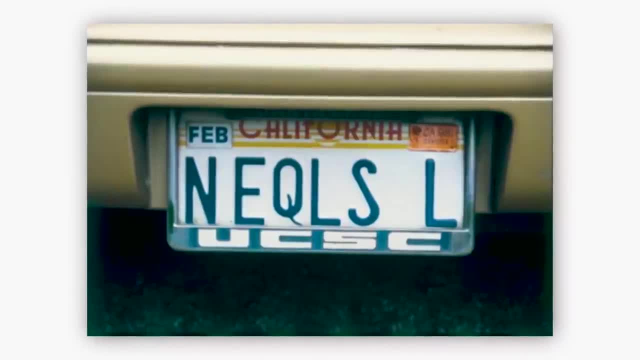 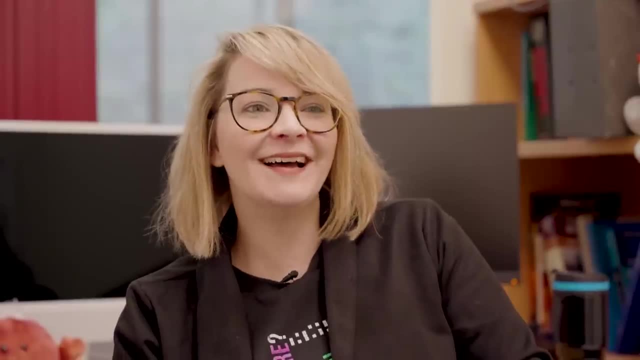 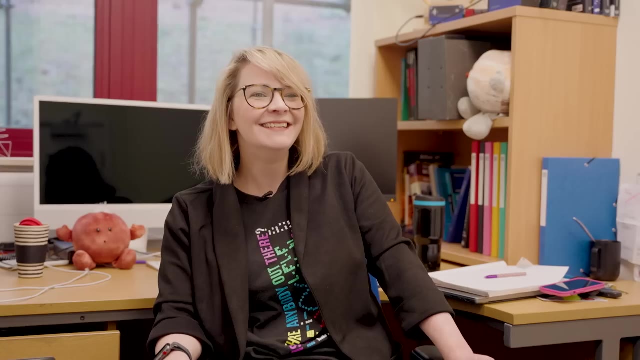 was n, eq, l, l, n, equal l. it was his number, and I have met three people with it tattooed on them. that's what I know of. I have also met a couple with this tattooed on them. yeah, yeah, I've not got any tattoos. okay, you've taken away my next question. let me ask you this then. all right, we've talked. 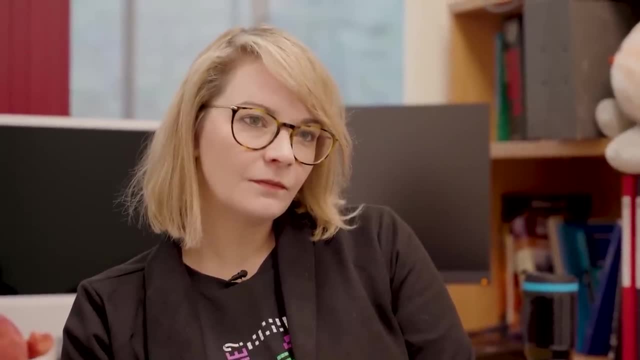 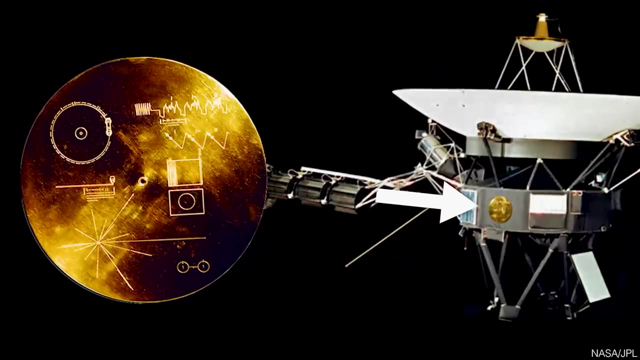 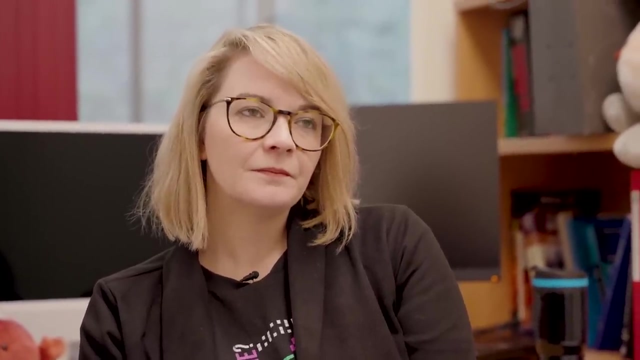 about listening, eavesdropping, trying to hear a message. another thing we obviously do is send messages. we've sent a couple of physical ones, bolted onto- yeah, Voyager, Voyager and things like that, yeah, but we've also, besides accidentally sending out- I love Lucy, we have deliberately sent. 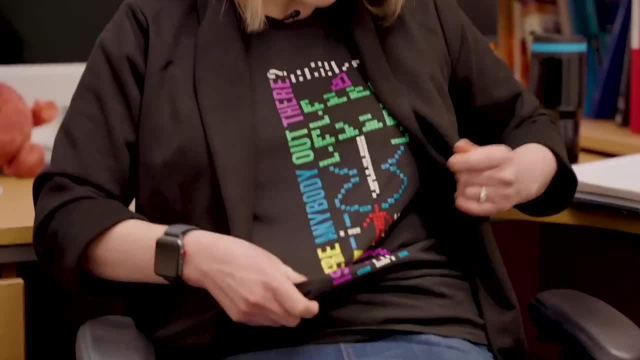 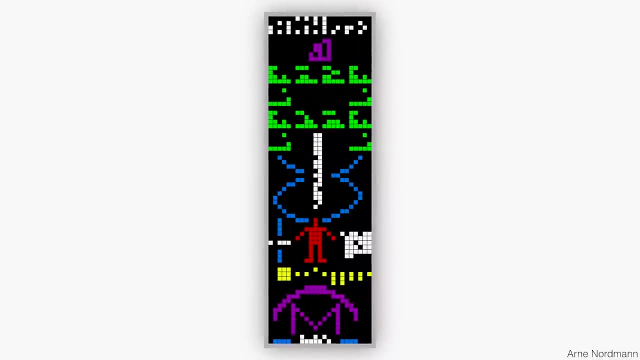 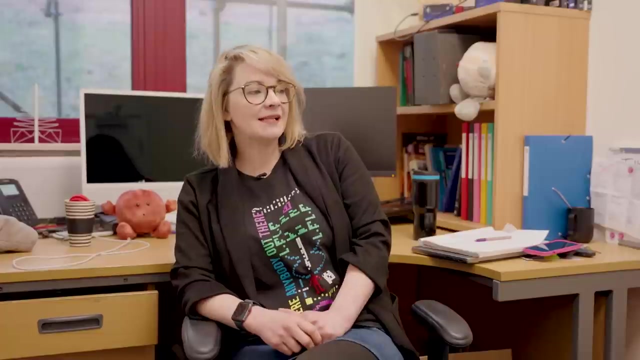 yeah, messages your t-shirt, yeah. so this is the only one that that has been sent out with any kind of real possibilities. i guess this was the drake message. so, frank drake, he happens to be the director of a really big radio dish called arecibo. he renovated it and in 1974 he was like, oh, we need. 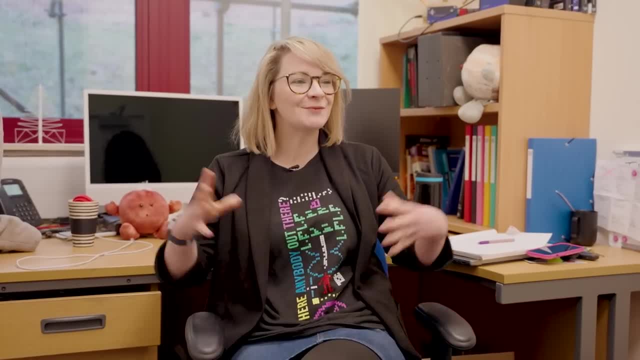 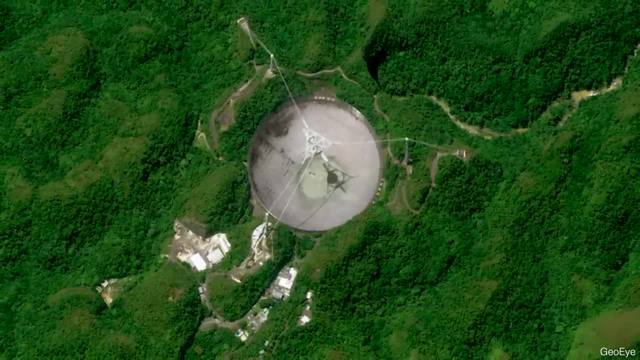 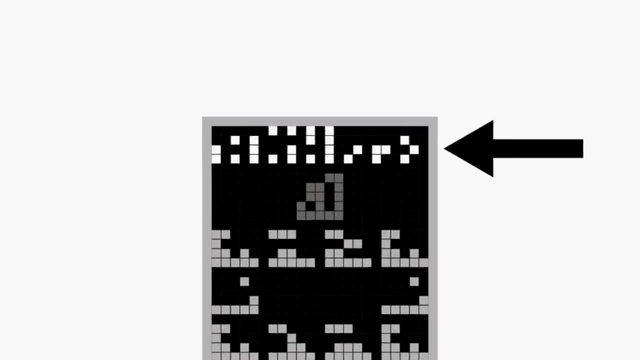 to make a big splash. what could we do? oh, and so what he did? he was invited everybody and he used this dish to send a really powerful radio signal in ones and zeros. and what this is? this is the base 10. so it's telling the civilization that we work in 0, 1, 2, 3, 4, 5, 6, 7, 8, 9, 10 in binary. that 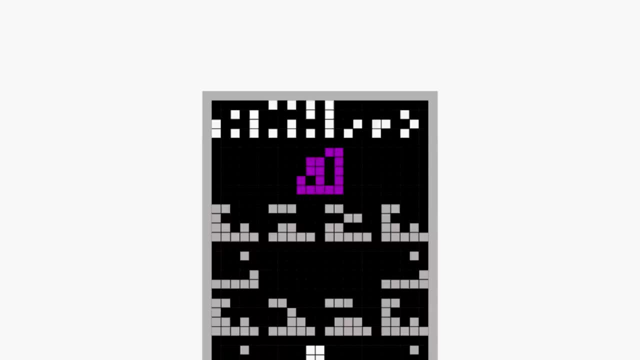 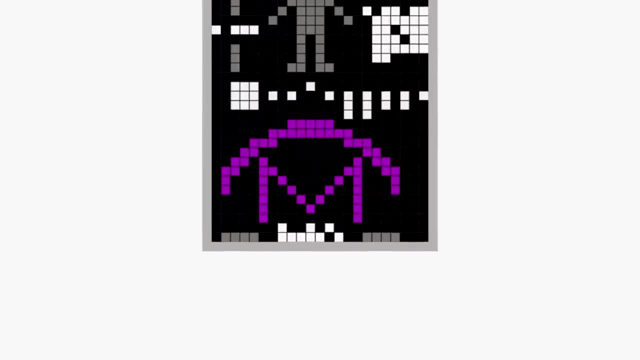 oh my gosh, i think that's some of the chemical elements that create dna. these are nucleotides. you've got a dna helix here. you've got a little person just here. this is our radio dish. this is arecibo. yeah, and you can, you can look up all of these. things mean, i love the little person. 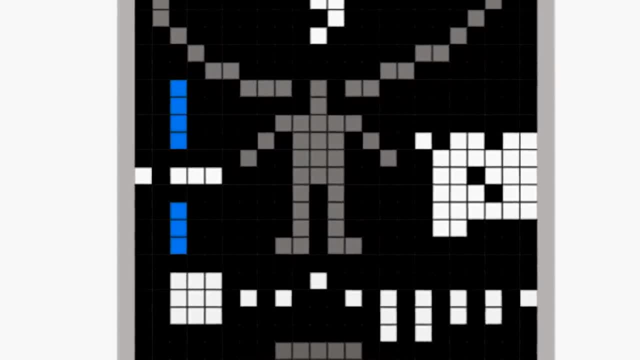 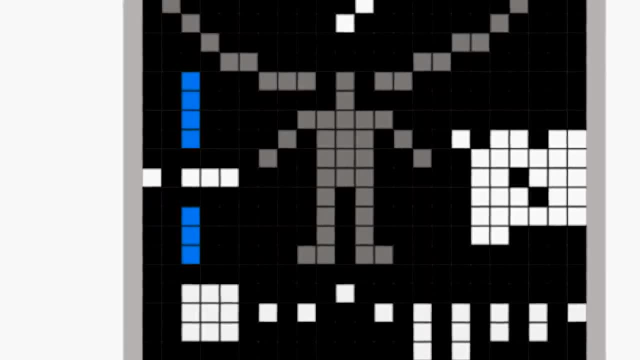 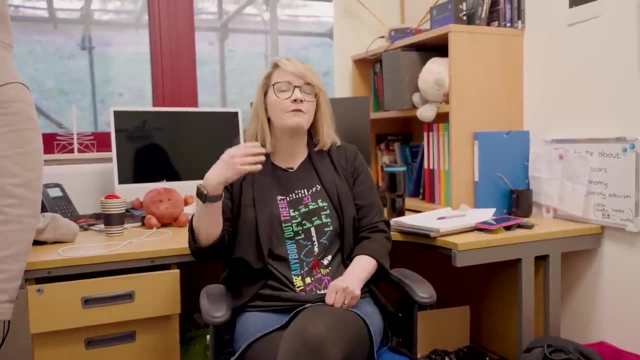 this is the dimensions of a human. i believe it's in units of 21 centimeters, which is like a really common radio wavelength that hydrogen emits, and so everything's done in 21 centimeters. because if you think we say, oh yeah, humans like 1.6 meters tall, what's a meter? um, but everybody knows what the spin, flip, transition of. 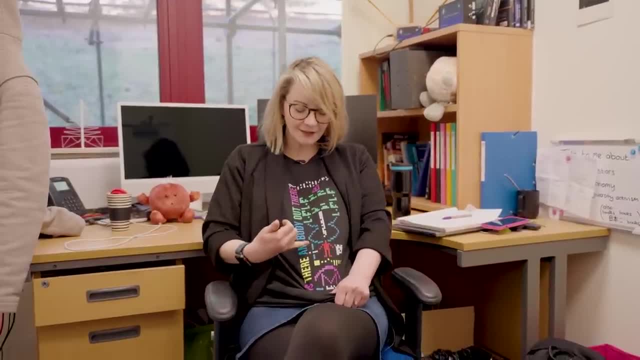 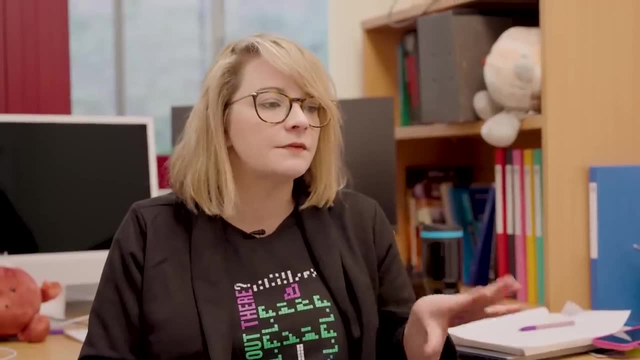 hydrogen is, that's 21 centimeters. so everything's done like a human's. this many of that, this, this size. are you happy with that message if you were the boss? i think it's nice and scientific. it's nice and calm it's also i think it's it's never going to get heard because it was more of a publicity stunt. 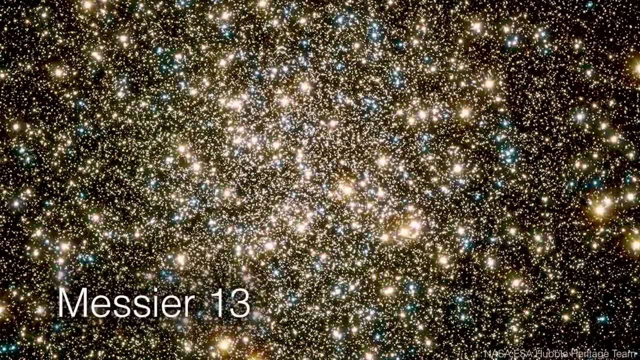 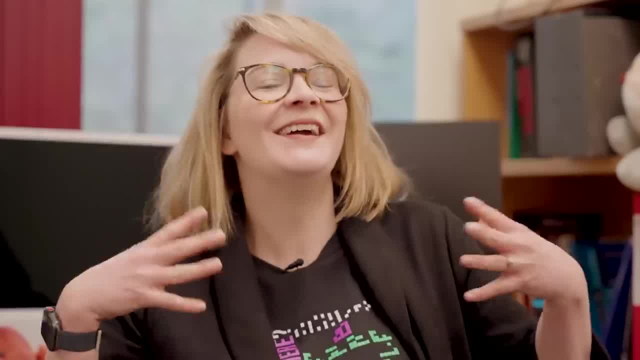 he sent it with huge power towards a specific galaxy, um. but the problem is that that galaxy is so far away that by by the time the message reaches it, it's actually going to have moved. so it was very much a publicity stunt. but we've sent so many radio communications out. i'm kind of 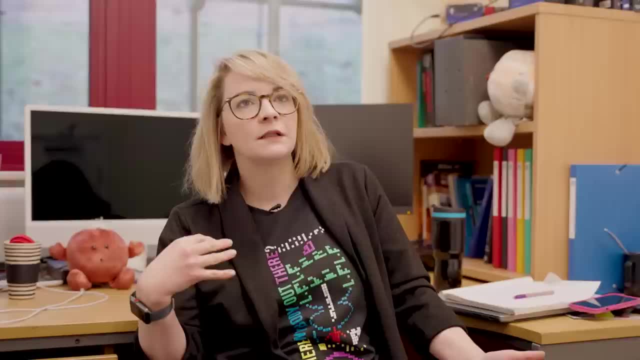 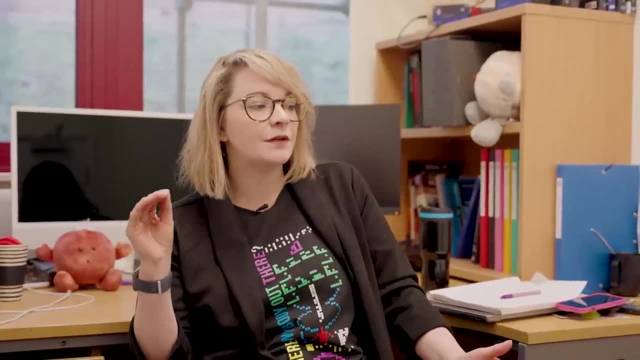 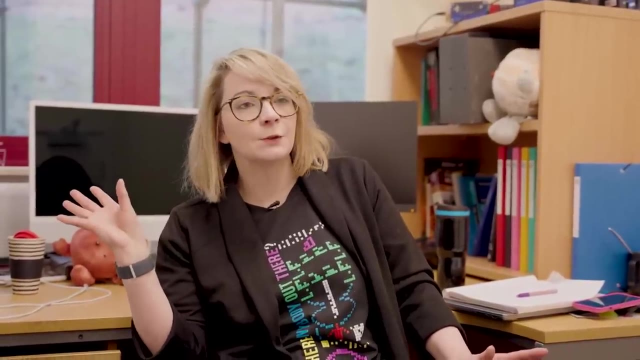 calm about sending more out, because i think that they've heard us anyway. if they're out there and they're out and about, so everyone's going to be surprised and going like, oh wow, it's a huge number of people, so what does that do to this galaxy and why is it so big? if it's it's so big? 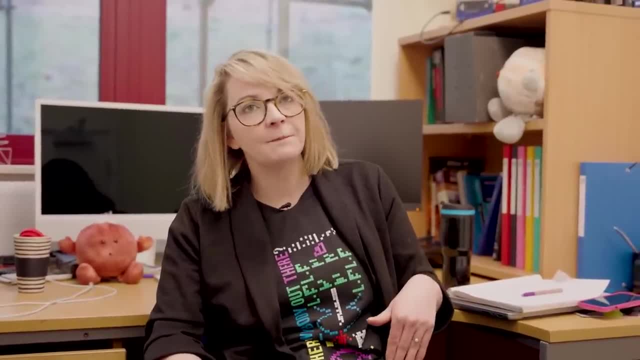 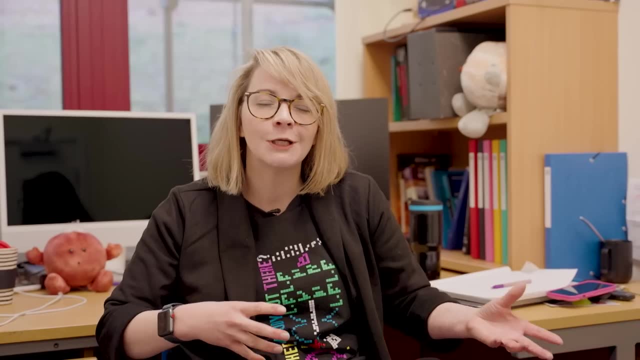 so i know if this doesn't work for life, i know if this doesn't work for us and it doesn't work for people. so we want to be prepared for future seasons for that. so i think we need to really know about it. and how do we predict that there's going to be a future of the galaxy in the future? and i think we need to pick up that right and we have to get it up and moving. that's what all of us are going to be doing and that's why we do this, and we'll see if we need to do it again, and we'll see. 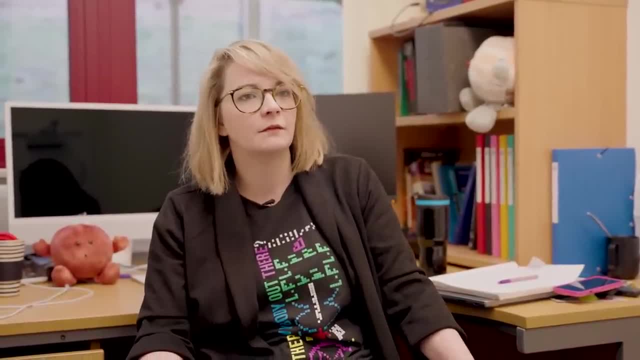 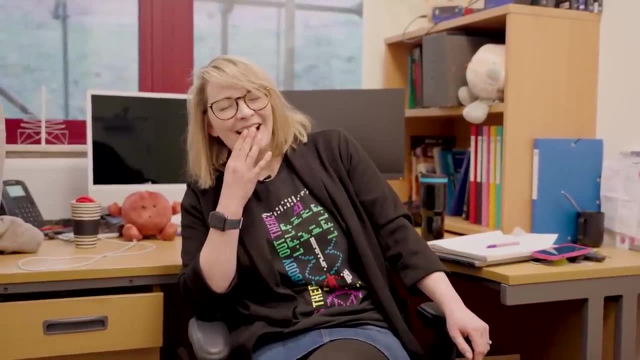 whether or not we can get it going at all. so yeah, we're still at that time, so we'll get your picture in the to happen. and why would they come? i mean, we're not great, all right, all right. well, you, i'll finish with this. then i know you've read the three body problem and i've read the three body problem and 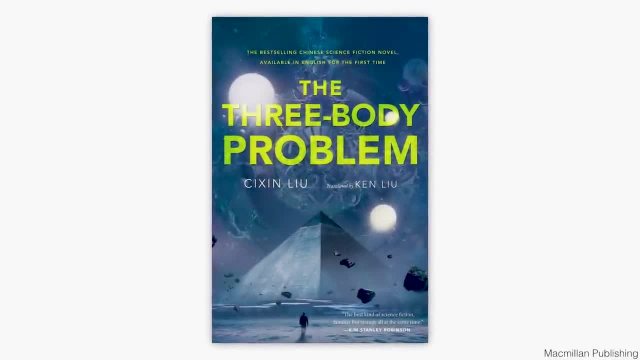 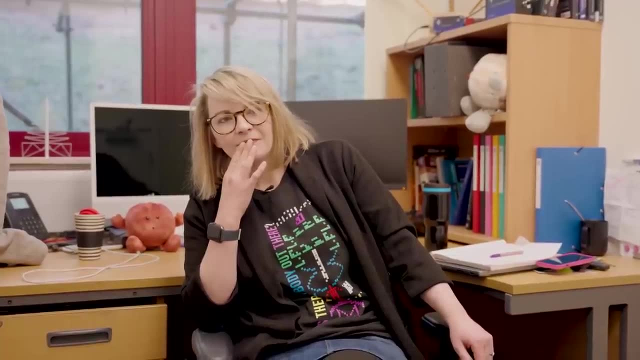 anyone who's read that knows there is a suggestion that we shouldn't stick our head above the parapet. you should just keep quiet. in that book, even without spoiling it, you don't necessarily even have to be able to visit a planet or a place to know there's life there and dispatch of it. 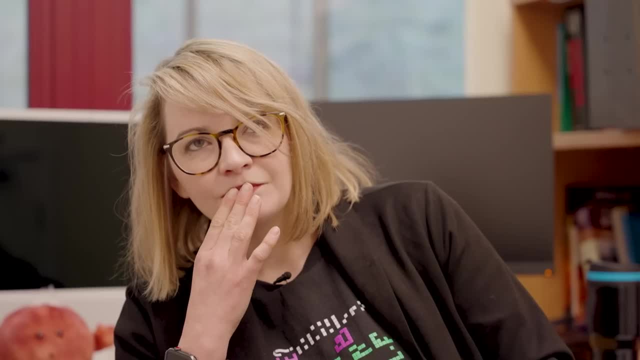 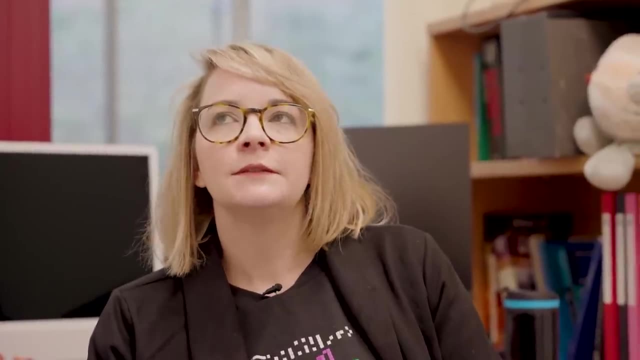 perhaps does that not scare you, does that not make you think we should be, we should be shutting up. oh, i'm just scared of everything. there's so much to be scared of on our planet that i kind of that's down the list of the things. i mean the three body problem, that is, there were so many. 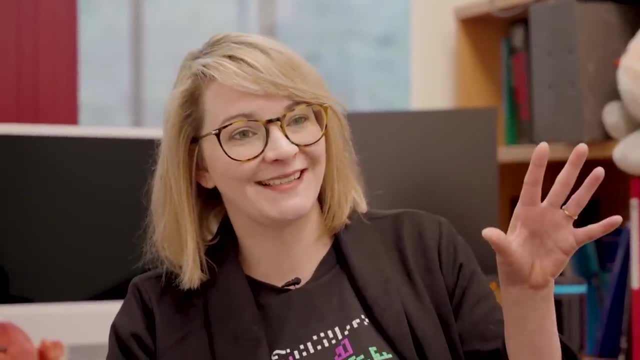 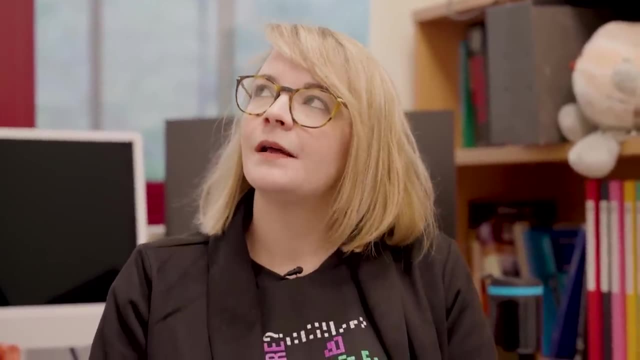 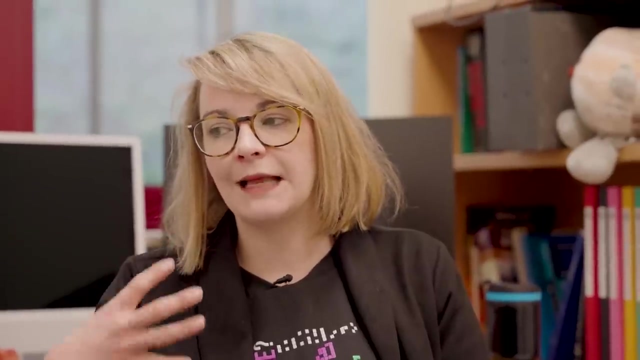 copies on the bookshelf in the- uh, the breakthrough listen labs that i went to in berkeley. it's all there, um amazing. there are scientists, um stephen hawking for example, who have spoken out very loudly to say: my god, we need to be quiet because otherwise we're just 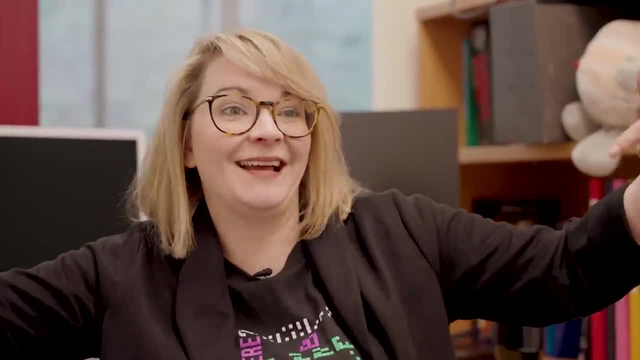 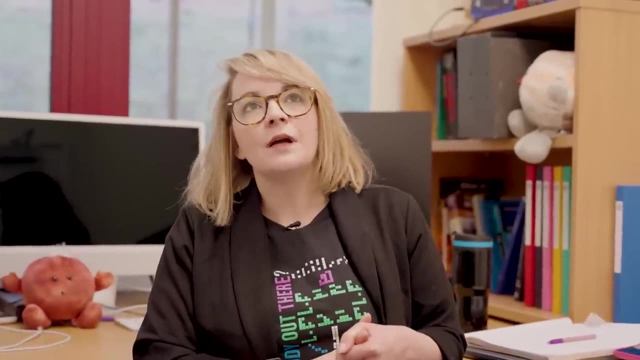 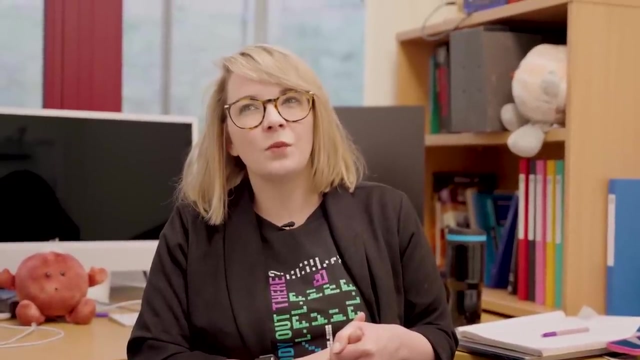 advertising to the universe: come eat us. we're here, having read frank drake's take on it in his excellent book, um, i would. i would say that it's. it's just so unlikely that they'd be able to visit and so unlikely that they'd want to take us over. i just, i just can't see it. i just can't see it. 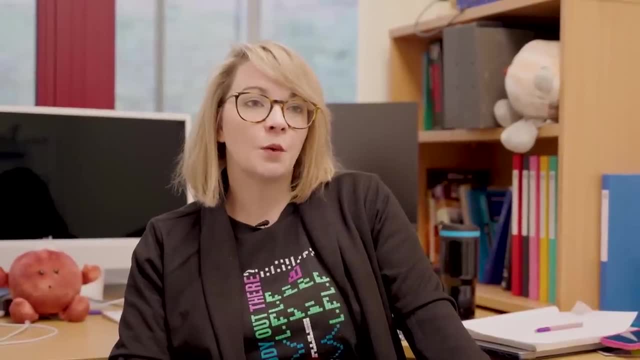 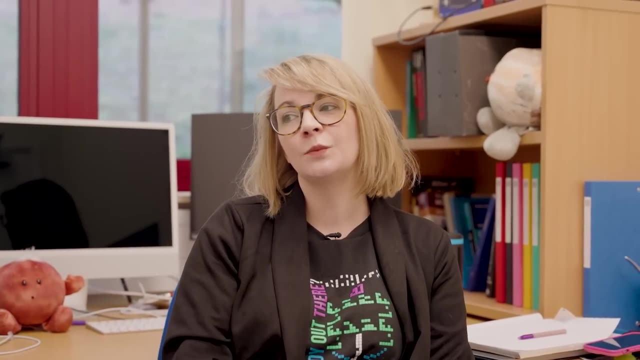 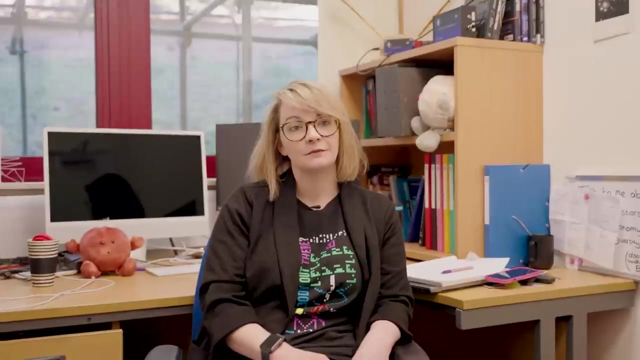 happening, and maybe maybe it's just i'm too scared of climate change to worry about the aliens at the minute. i'm not sure, but i kind of see it as like: look, we've already done it. yeah, it's already out there. to kind of encapsulate the argument. as i understand it, though, the argument is: 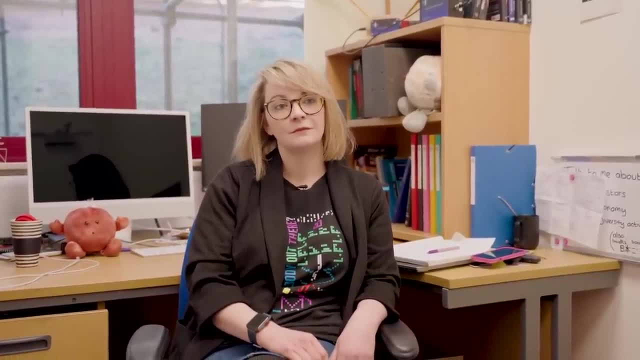 like if you walked into a forest and every single creature and everyone was being absolutely quiet and you weren't hearing a peep, and you walked into that forest. you might think, well, maybe i should go to the forest, and i should go to the forest, and i should go to the forest and i should. 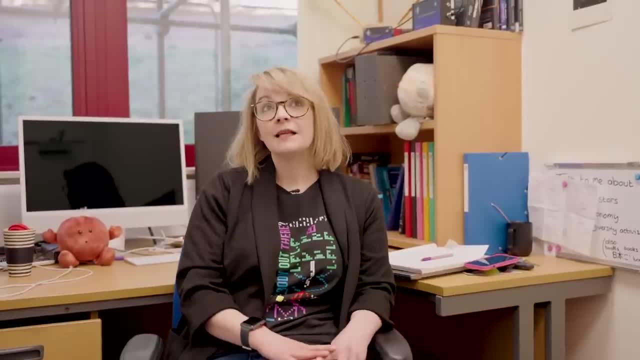 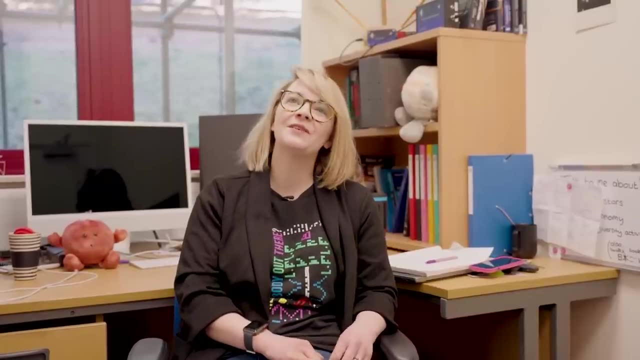 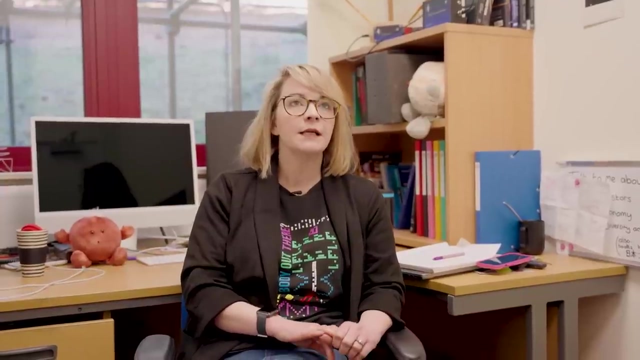 be quiet too. maybe there's a reason everyone here's been quiet, and definitely the third book of the third body problem, um, definitely made me pause in terms of of that, i and, yeah, the idea is that you probably should be quiet, right, you should be cautious, but we can't stop for us to do that.